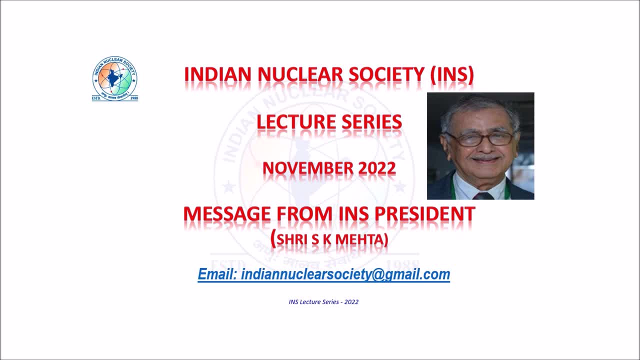 in various areas benefiting humanity, the limitations and the regulatory aspects in safety and protection. One of the main objectives of the INS is to promote the advancement of nuclear science and engineering and technology related to the atomic energy. With this objective, INS has been disseminating information through journals, books, reports. 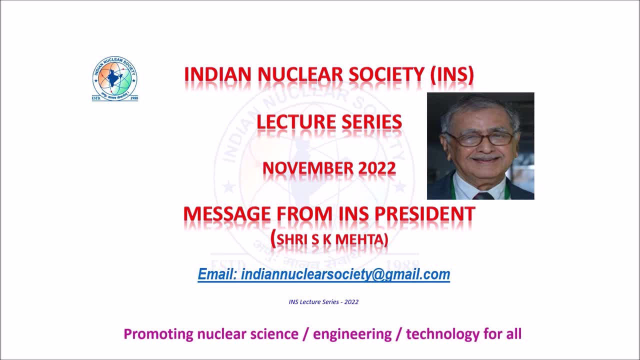 newsletters, seminars and conferences. These have mainly been to keep the INS members and other scientific communities and organizations well informed about the development in the various areas. Thank you. This is an opportunity to discuss the importance of nuclear science and engineering and the importance of science and technology within India and the world over. 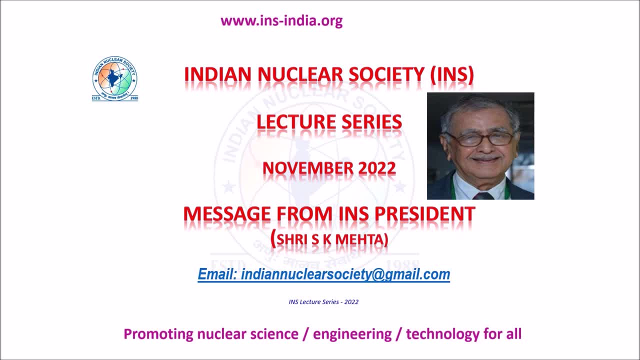 Already realized that there is a need to keep the various professionals, undergraduate students and general public knowledgeable in the respective fields of nuclear science and engineering For the benefit of the public. some of the patent and the common application of nuclear being for power, industrial use, medical diagnosis. 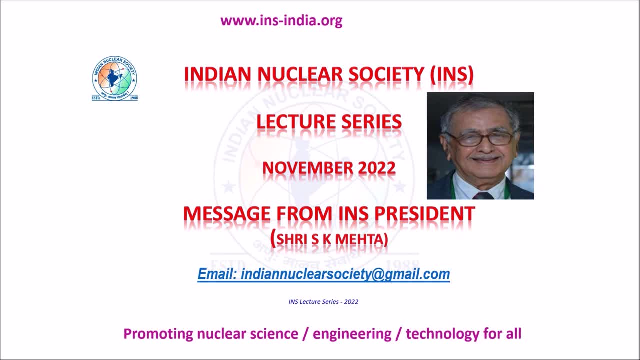 and treatment, agriculture, food preservation and various other areas. This lecture series is made in simple language and illustration with the aim to inform the general viewer about the science, engineering and technology. social benefits of the nuclear application, of nuclear carrier, benefits in nuclear and regulatory and safety of the. 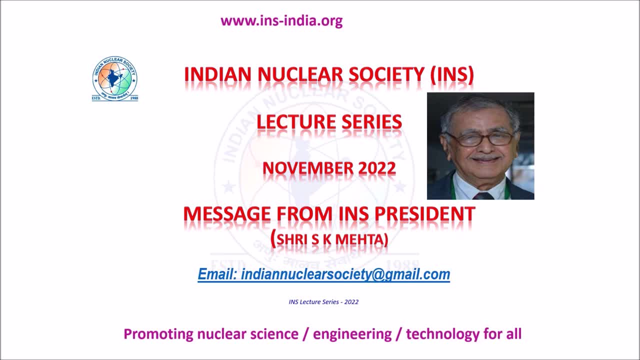 nuclear energy. The presentations are prepared and narrated by experts on each topic in a way that the viewers with no background knowledge about the nuclear science and engineering can understand. Our effort will be to constantly provide information about newer benefits to the society emerging out of the pain-taking research and nuclear 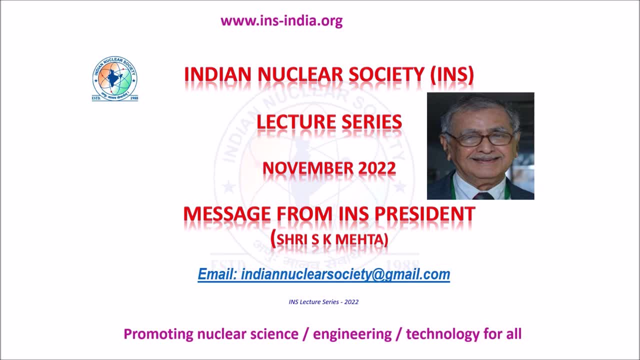 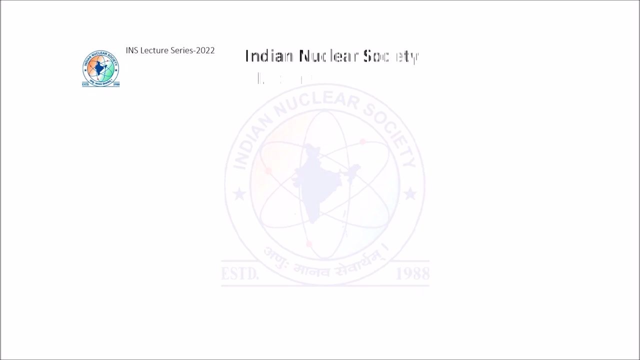 science and engineers. Viewers are encouraged to comment, suggest and put forward questions to the experts. The channel of constructive communication will always be open in INS, which is a website of INS. Welcome all to this wonderful lecture series by Indian Nuclear Society. 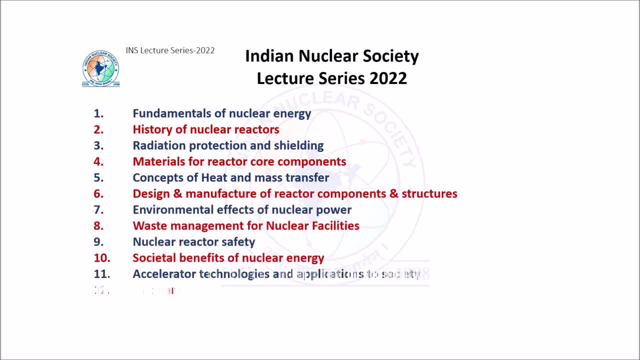 There are 13 lectures on various topics related to nuclear energy and its application to societal benefits. All these lectures will cover different aspects of nuclear energy in sectors like power energy power medicine, agriculture and society. It illustrates in simple way the science behind nuclear reactors for all of us. 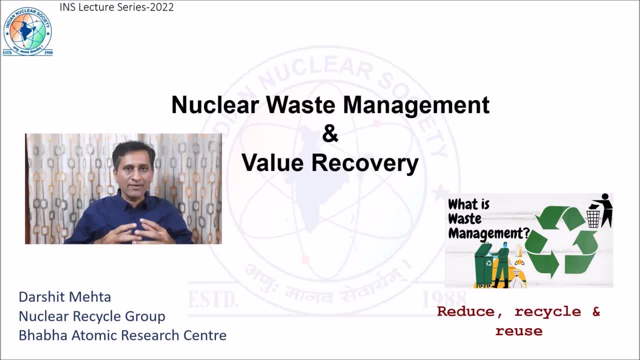 Hello friends, welcome to the INS lecture series 2022.. This lecture is about management of nuclear waste and value recovery. We all know that every industry generates one or other type of waste which needs to be managed safely and efficiently, not only to protect the public and environment, but 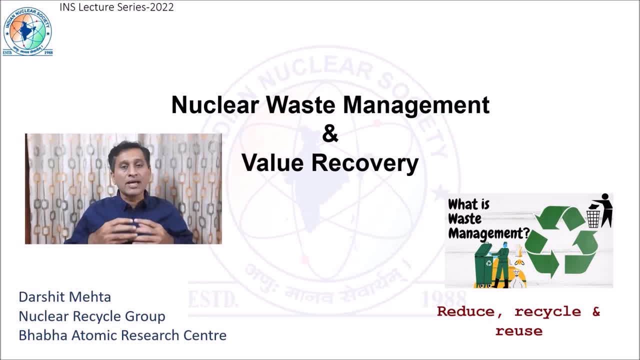 also to protect the environment. These lectures are designed to improve the cost optimization, economy and sustainability of the particular industry. Nuclear industry is also not apart from that. While generating electricity using nuclear energy, it also generates various types of waste which needs to be managed safely and efficiently. 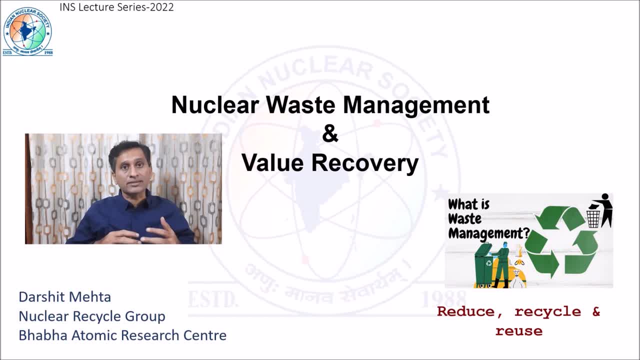 So this lecture is an attempt to present the strategies and practices being followed for the safe management of nuclear waste, along with the scientific and technical facts. The lecture is mainly focused on the following. In this lecture we will discuss the following: focus on the management of nuclear waste arising from the pressurized heavy water reactor. and. 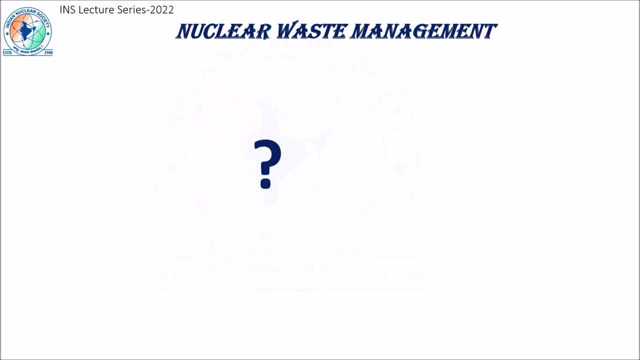 associated fuel cycle activities. Let me start the lecture with a general perception about nuclear waste and its management. Whenever we think about the nuclear waste and its management, there are various questions arising in our mind, such as what will be the amount of waste, How they are managed. 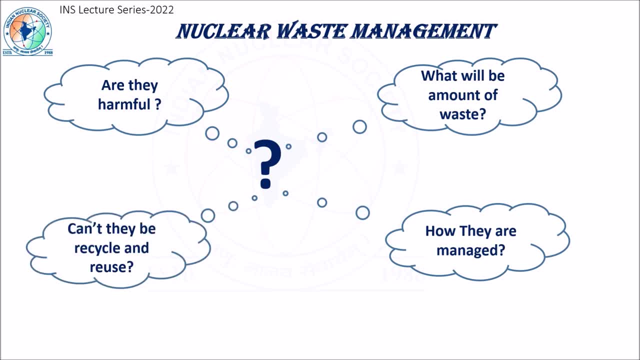 Are they so harmful? Can't they be recycled and reused? or can't we convert the nuclear waste into the wealth? Such various questions are always be present in our mind. Let me present the strategies and practices being followed for the safe management of nuclear waste, and I am sure that by the end of this lecture various such questions will. 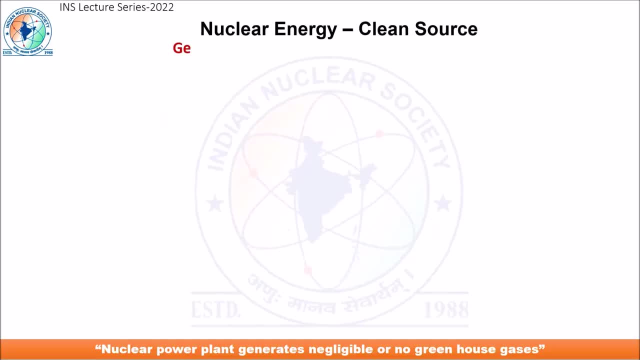 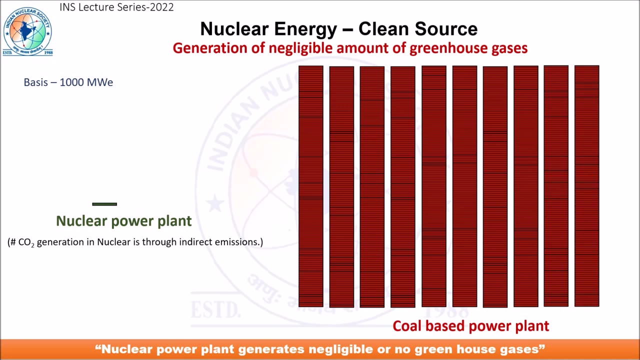 be amicably addressed, Catching upon an important feature of nuclear energy, that it's a nuclear power plant. it is a clean source of energy. The nuclear power plant generates negligible amount of greenhouse gases, while generation of the electricity as compared to those are getting generated from coal based power plant. 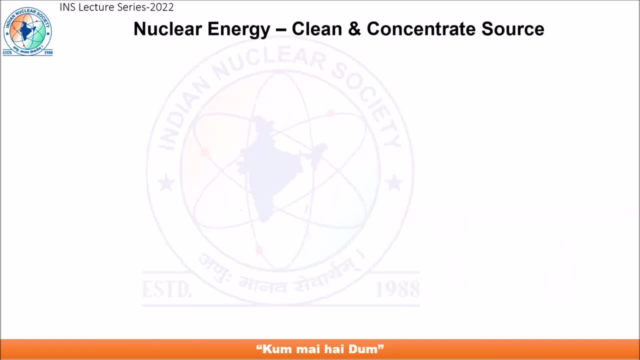 Besides this, nuclear energy is also a concentrate source of energy because it is a large energy density system and hence it requires lesser amount of fuel for production of electricity. For example, one gram of uranium-225 can generate energy. One gram of uranium-235 can generate energy. 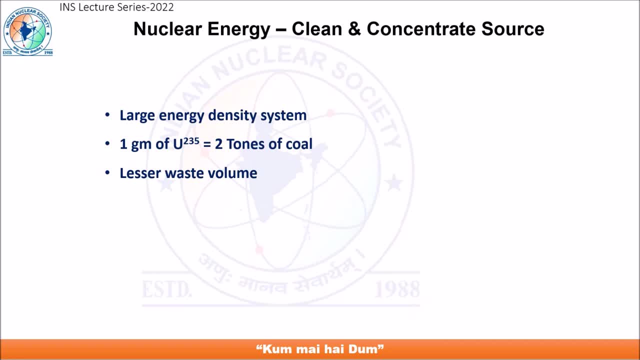 One gram of uranium-235 can generate energy. One gram of uranium-235 can generate energy. As much as that can be extracted from equivalent two tons of coal, So the lesser fuel is required. hence it also generates lesser amount of the waste volume. 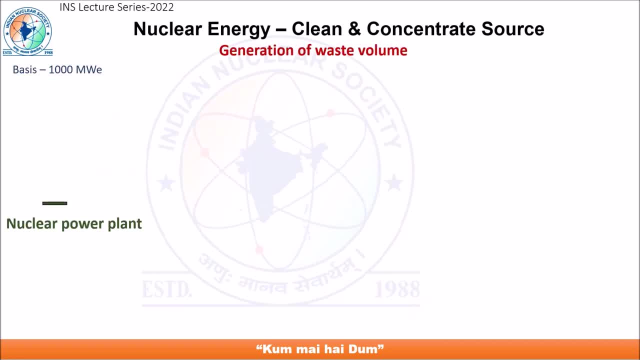 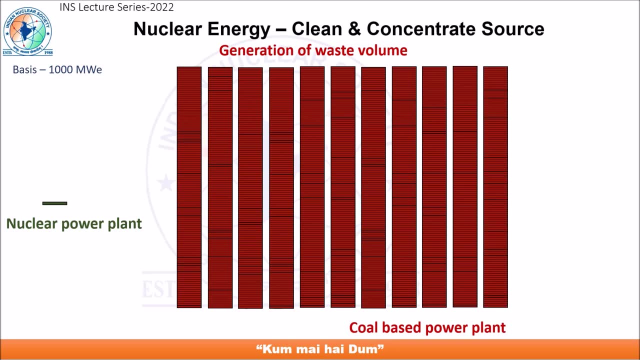 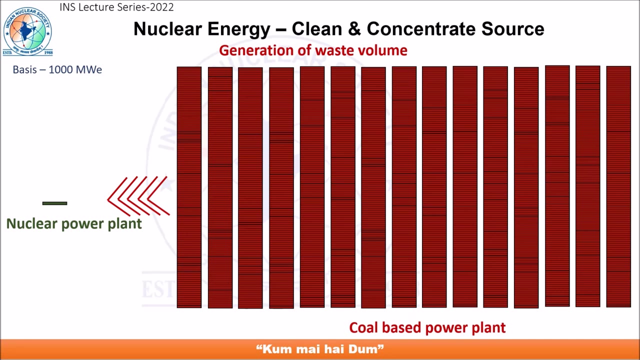 Or during the operation of the nuclear power plant for production of the electricity. the overall waste volume getting generated from nuclear power plant is much, much lesser as compared to those getting generated from coal based power plant, And it's really true for nuclear energy. that come mayhe dum. 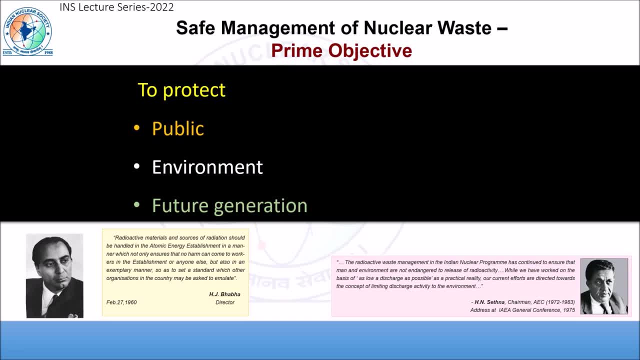 However, whatever small quantity of nuclear waste is getting generated, it needs to be managed safely and efficiently to protect public environment, future generation and also to improve the economy and sustainability of nuclear industry. As a result, safe management of nuclear waste has been accorded highest priority since inception. 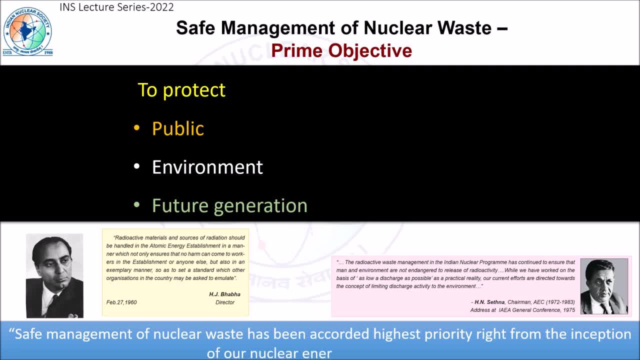 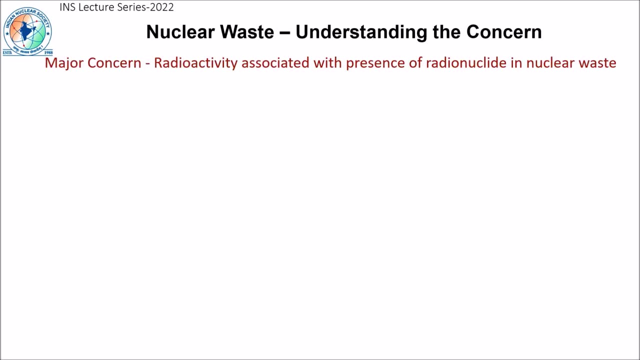 of nuclear power program in India, The strategies and practices for safe management of nuclear waste have been drafted and put in practice in such a way that waste do not adversely affect the public and environment. Before touching upon the strategies and practices followed for the safe management of nuclear 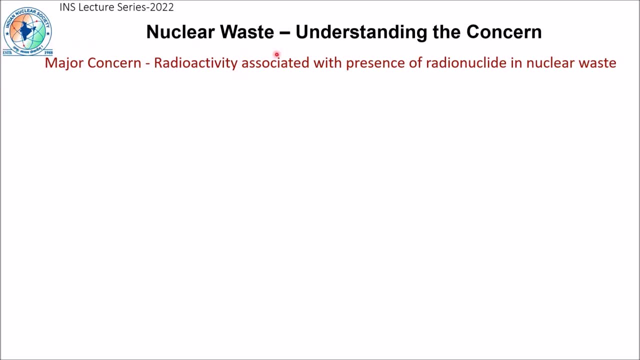 waste. let us try to understand the major concerns associated with the nuclear waste. These concerns are mainly due to the radioactivity which are associated with the presence of radionuclide in nuclear waste. Nuclear waste may contain different types of radionuclide and we all know that radionuclide 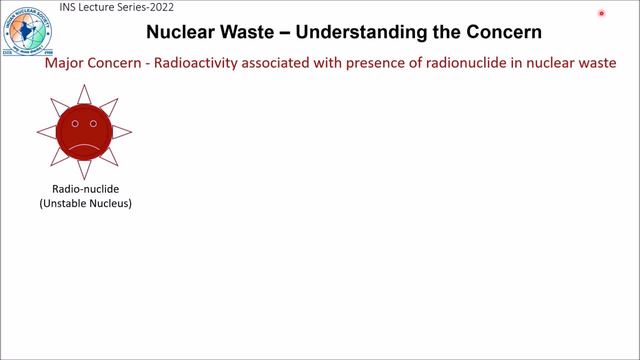 is an unstable nucleus. It is unstable in nature because it consists of higher energy than what it requires for its stability. As a result, after some time, this unstable radionuclide decays two-thirds to one-third of its energy. This unstable radionuclide, with emission of its additional energy, either in form of alpha, 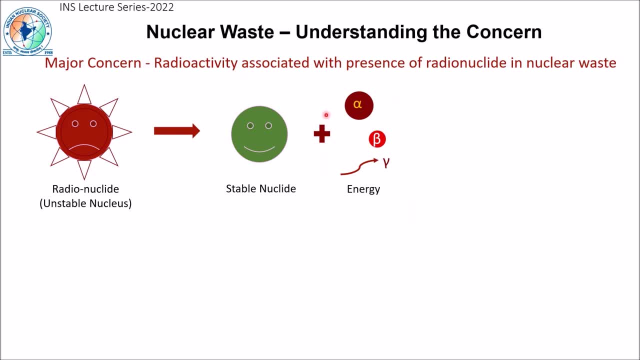 beta or gamma radioactivity. It is this energy or radioactivity whose effect to the public and environment makes the major concern for the nuclear waste. But nuclear waste has one very important feature: that the radioactivity and its associated hazard potential of nuclear waste reduces with time. 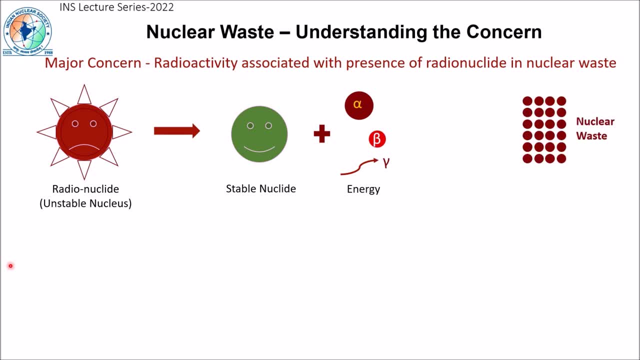 Now let us understand how. Suppose we have a nuclear waste with certain number of radionuclides. As time passes, the radionuclide decays to the stable nucleid. As a result, with passage of time, the number of radionuclides present in nuclear waste. 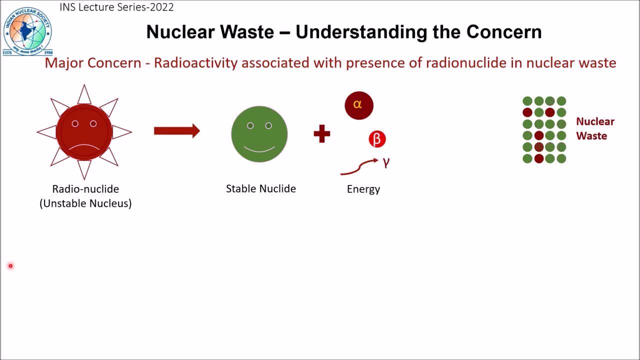 reduces and hence radioactivity and associated hazard potential also reduces. If we plot the graph of hazard potential of nuclear waste, we can see that the radioactivity and associated hazard potential of nuclear waste are reduced. We can see that the hazard potential of nuclear waste reduces with time. 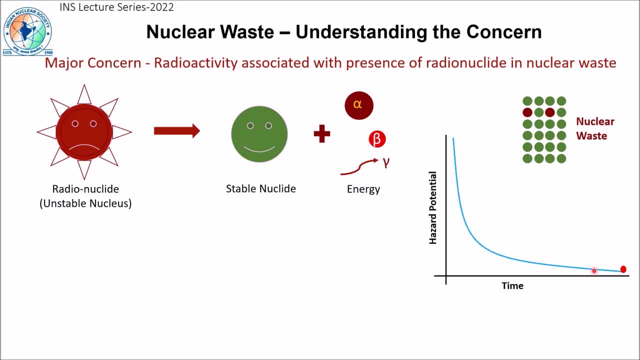 And the time will come where the hazard potential of nuclear waste reduces to such a low level that the nuclear waste will not be harmful to the public and environment. We must know what is that timeframe, and that depends upon the half-life of radionuclides. 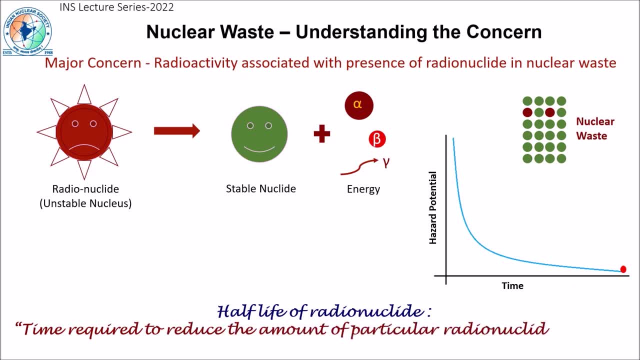 present in nuclear waste. So this is the time frame, Suppose we isolate the nuclear waste and allow the decay of the radionuclides present in nuclear waste for a time frame of about 10 half-lives of the radionuclide, the radioactivity. 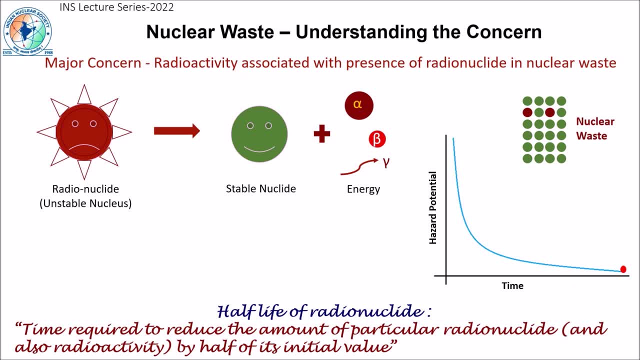 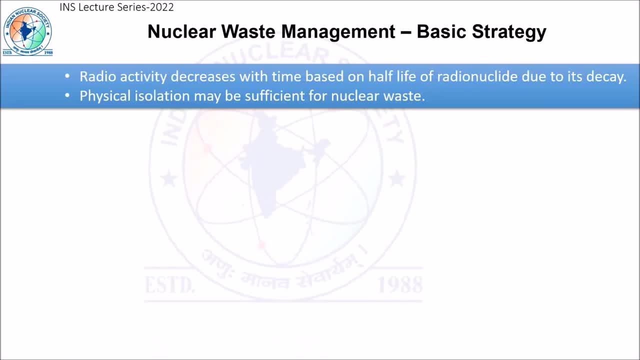 and its hazard potential of nuclear waste can be reduced by 1000 times as compared to its initial value. This feature of nuclear waste is very important for drafting and finalizing the strategy for its management. Suppose we have a nuclear waste which contains the radionuclide having very short half-life. 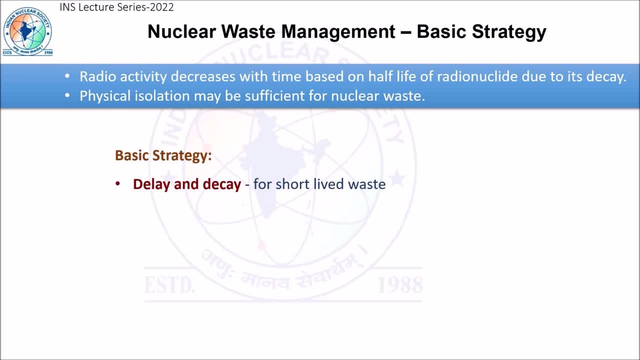 then we require shorter time period, time frame for allowing the decay of majority of radionuclides present in the waste, so that the waste becomes very, very low active and will not be further harmful. In such cases, we follow the following procedure. We follow delay and decay strategy, where we deliberately delay the processing or treatment. 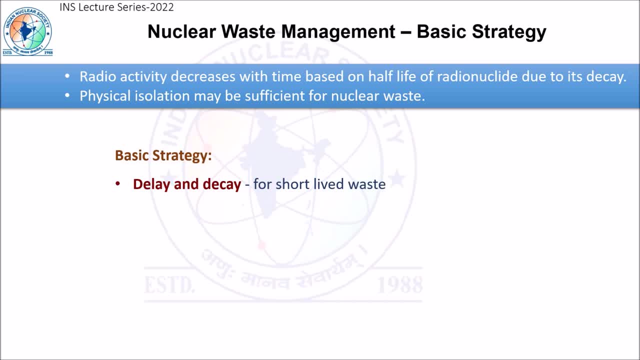 of the waste and allow the majority of radionuclides to decay so that the waste becomes very, very low active and can be further processed as an inactive material. Suppose our waste contains very low amount of the radioactivity, then we follow: dilute. 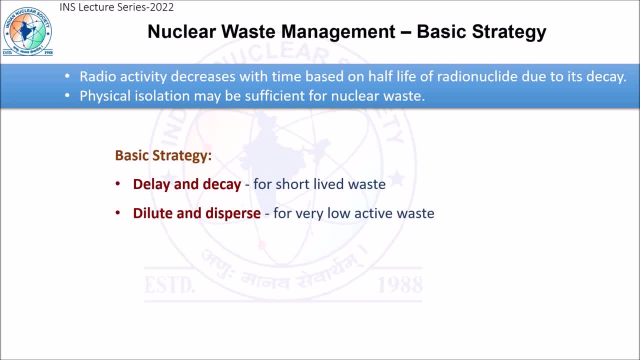 and disperse strategy, Where we follow the following procedure: We dilute our waste with sufficient amount of inactive element to bring down the radioactivity level of the waste below the limit prescribed by regulatory authority. So the waste is diluted in such a way that the hazards associated with waste becomes. 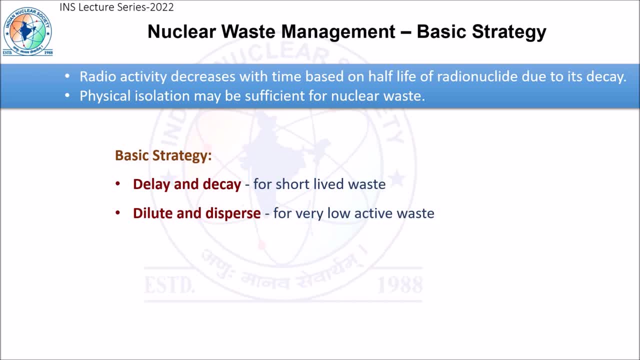 almost negligible and then it can be dispersed as a normal waste. But suppose we have a waste which contains appreciable amount of the radioactivity and the radionuclide also consists considerably medium or long half-life, then both the above strategy cannot be used. 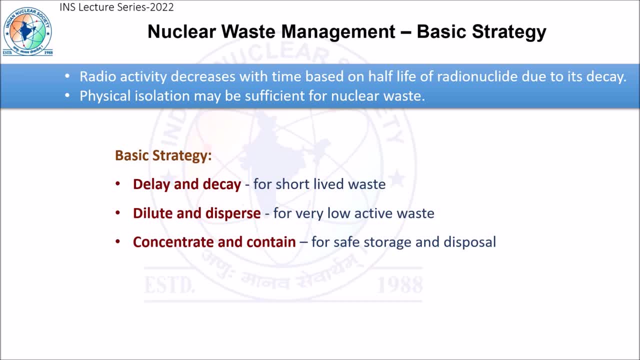 And we need to follow concentrate and content strategy, where we concentrate the entire radioactivity in smaller volume And then contain them in such a matrix so that the migration of radionuclide can be minimized to very, very, very low amount. In subsequent part of our lecture we will discuss that- how the concentrated waste is. 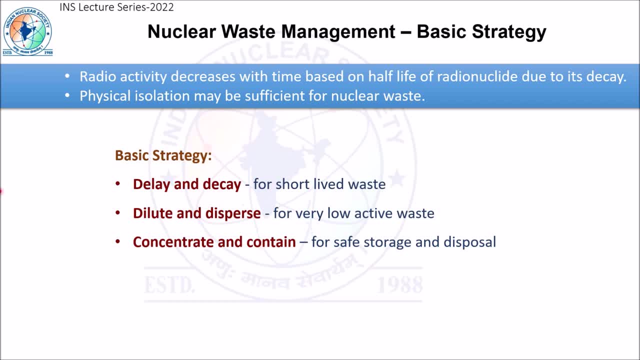 contained in an inert matrix so that the migration of radionuclide can be minimized to the negligible level. And in practice, we do follow single strategy or combination of two or more strategies. However, whatever the strategy we do follow, we must practice the recycle and reuse of 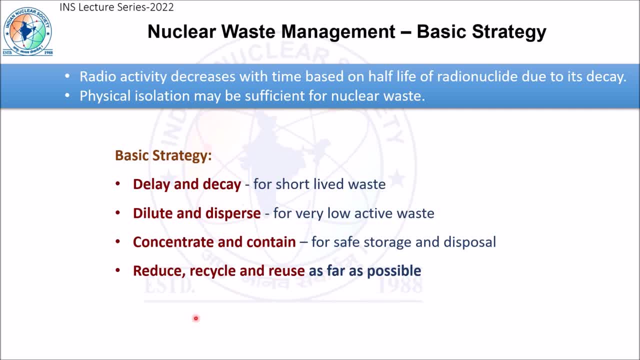 material as far as possible so that the waste volume can be reduced effectively, And in our subsequent part of lecture we will also discuss that- how the valuable material is recovered from nuclear waste And they are deployed either as a fuel for production of electricity or as a fuel for 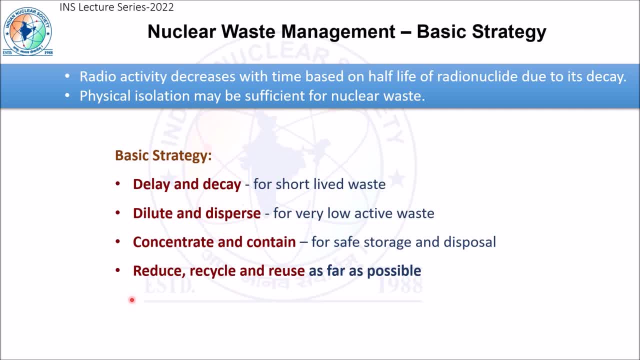 the production of energy, And in our subsequent part of lecture we will also discuss that, how the valuable material is recovered from nuclear waste And they are deployed either as a fuel for production of electricity or as a valuable radionuclide for various societal application, and which finally results in effective and 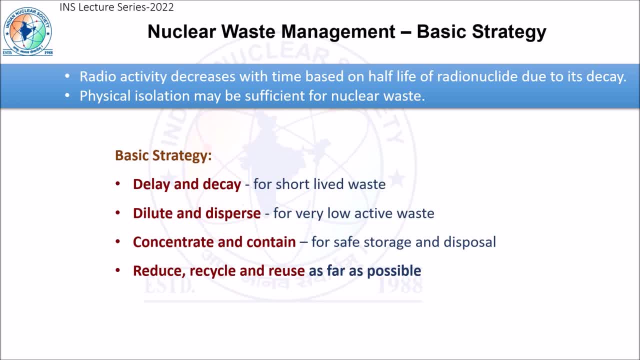 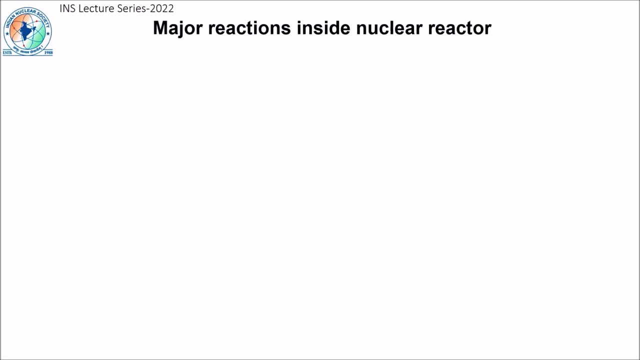 significant minimization of waste volume. Very important to understand the genesis of the radionuclide which makes the nuclear waste a radioactive in nature And, for the same, let us try to understand the major reactions taking place in the nuclear waste. If we take a case of pressurized heavy water reactors, or PHWRs, which are under operation, 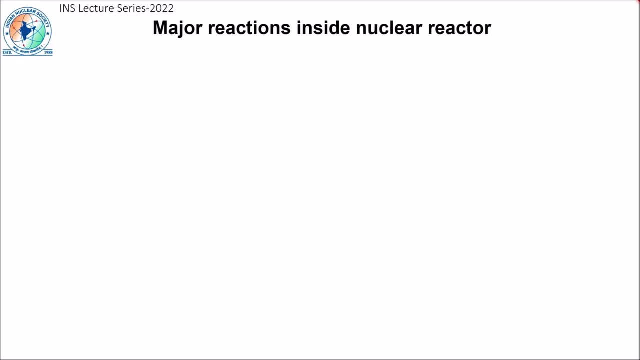 and contributes a major share of electricity from nuclear energy in India. We all know that PHWRs utilizes the oxide of natural uranium as a fuel, and natural uranium consists about 0.7% of uranium-235 isotope, while more than 99% of uranium-235 isotope 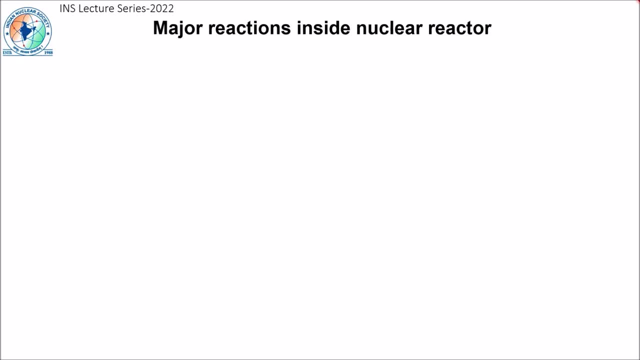 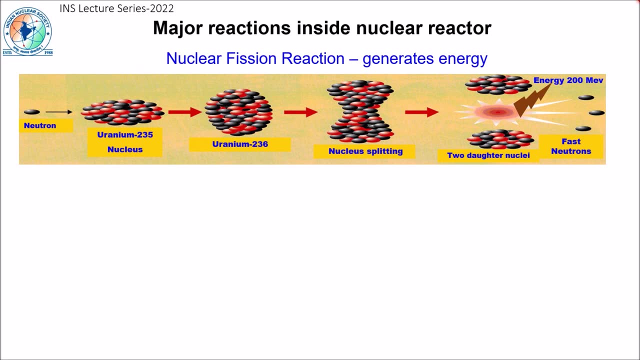 The most important nuclear reactions taking place inside the nuclear reactor is fission of uranium-235 isotope. Uranium-235 absorbs the neutron and gets fission into two smaller mass number nuclei and also generates the energy and two or three number of neutrons. 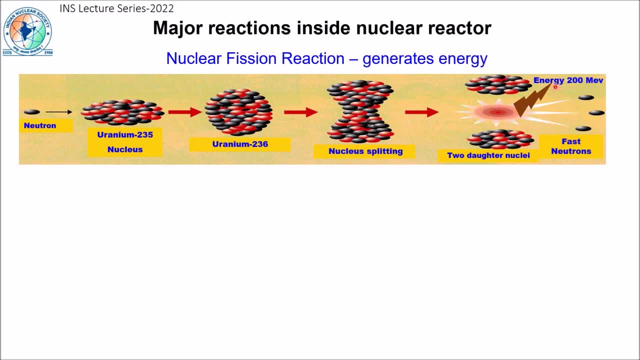 The energy is utilized for production of the electricity. The energy is utilized for production of the electricity. The energy is utilized for production of the electricity, While these two smaller mass number nuclei are usually called fission products because they are getting generated from the nuclear fission reactions. 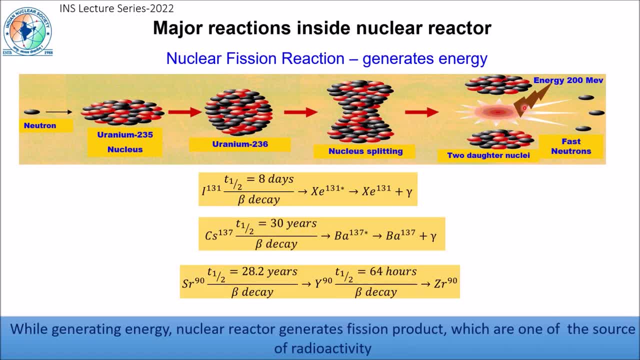 These fission products. when decays to their daughter product, they generates usually beta gamma radioactivity and the fission products are usually short lived or medium lived, except few. So it is this fission products and their daughter products which contributes significantly or which is the one of the most important source of 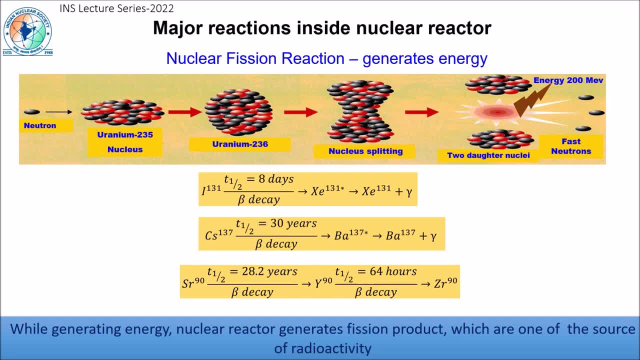 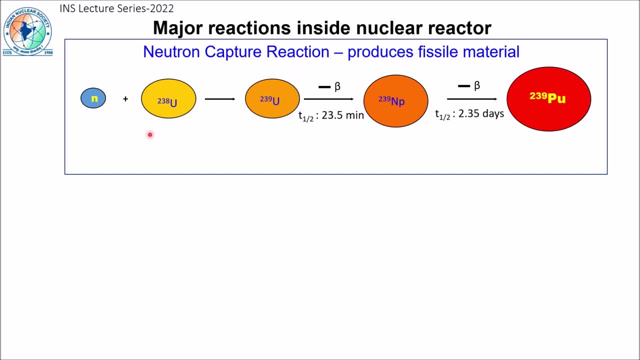 radioactivity in nuclear race. Another important reaction taking place inside the nuclear reactor is a neutron capture reaction. Uranium-238 isotope, which is largely available in the fuel, when absorbs the neutron, finally gets converted into the Plutonium-239.. This Plutonium-239. 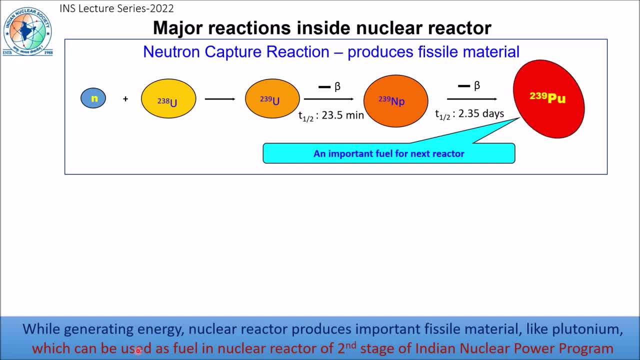 is one of the most important fission material and can be used as a fuel in nuclear reactor of second stage of Indian nuclear power program for production of electricity. Some of these Plutonium-239 nuclei further absorbs the neutron and finally gets converted into the higher mass number actinides. 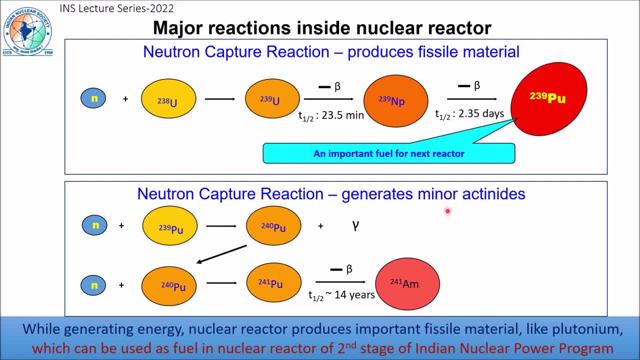 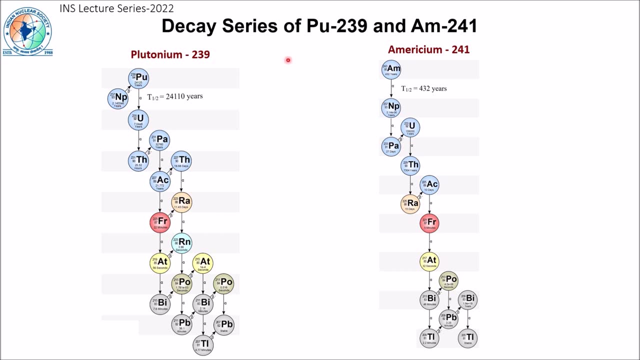 These higher mass number actinides are usually called as a minor actinide. Ambrosium-241. is one of the prominent minor actinide getting generated due to such neutron capture reaction. Thus produced Plutonium-239 and minor actinides like Ambrosium-241 are also radioactive in 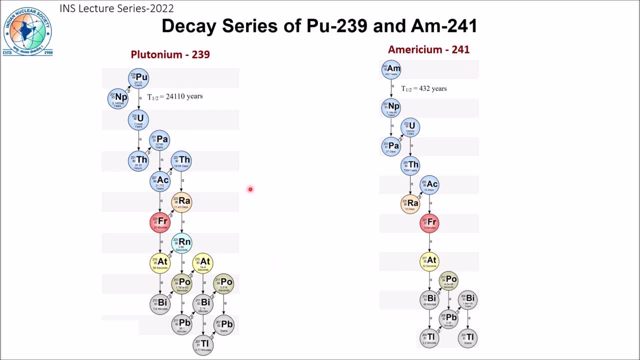 nature. They usually decay to the stable product by series of alpha as well as beta decay. Besides this, they are also usually long lived in nature. So they are usually decayed to the stable product by series of alpha as well as beta decay. Besides this, they are also usually long lived in nature. 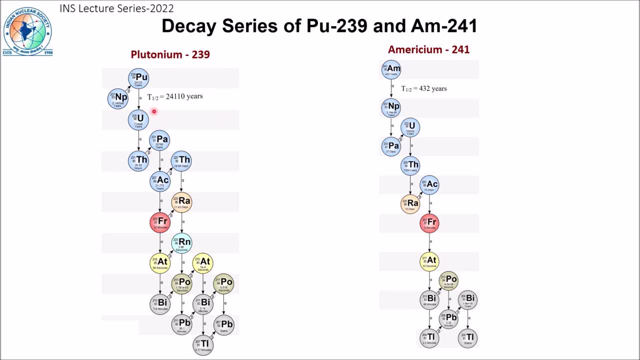 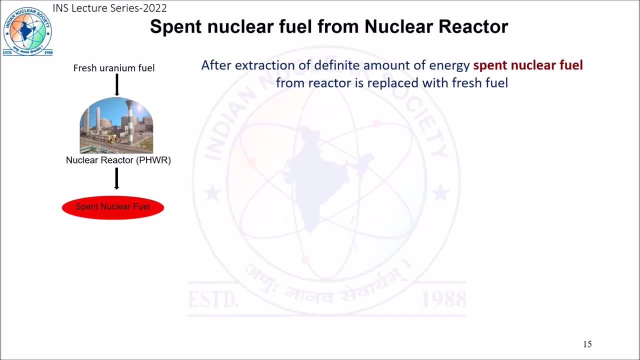 So they are usually long lived in nature. For example, Plutonium-239 has half life of about 24000 years, while Ambrosium-241 has half life of about 430 years, Due to these important nuclear reactions which are taking place inside the nuclear reactor. 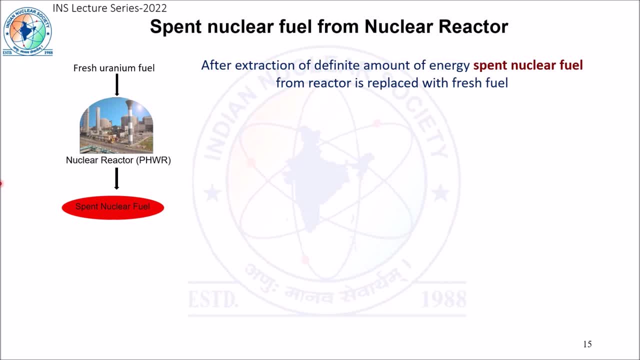 one side, uranium-235 isotope is getting consumed by nuclear fission reaction for production of energy. At other side, uranium-238 isotope is converted into the Plutonium-239 by neutron capture reaction. At other side, uranium-238 isotope is converted into the Plutonium-239 by neutron capture reaction. 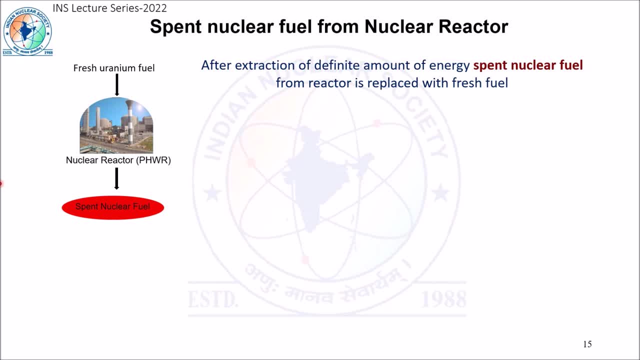 At other side, uranium-238 isotope is converted into the Plutonium-239 by neutron capture reaction. Thus generated radionuclides, including fission product, Plutonium, minor actinide, along with uranium, remains within the fuel inside the nuclear reactor. 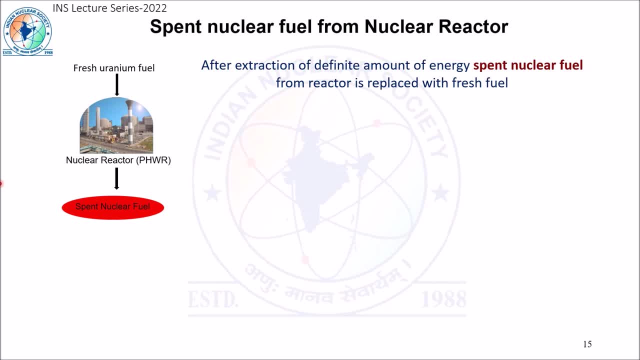 As uranium-235 is getting consumed by nuclear fission reaction, there will be a depletion of uranium-235 isotope inside the fuel. As a result, after extraction of definite amount of energy, the fuel has to be replaced with the fresh fuel for maintaining the sustainable fission chain reaction inside the nuclear 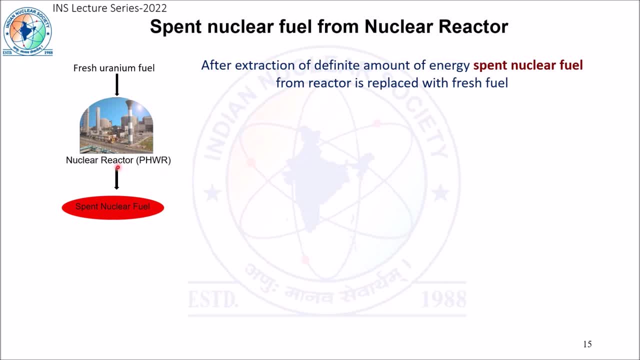 reactor. The fuel which are coming out from the reactor is usually called spanned nuclear fuel. As we discussed that nuclear energy is a large energy density system, it will require a lesser amount of fuel to be consumed for production of energy. If we take a case of PHWR, it will take hardly more energy than the amount of energy consumed. 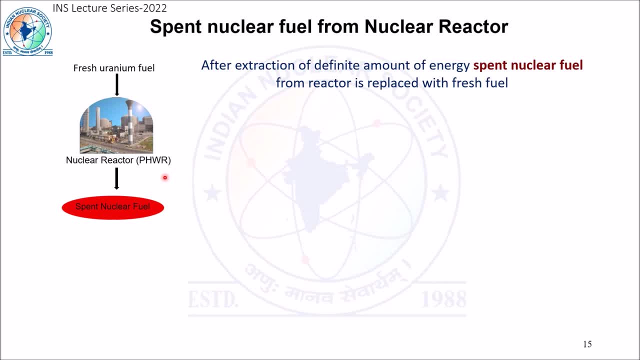 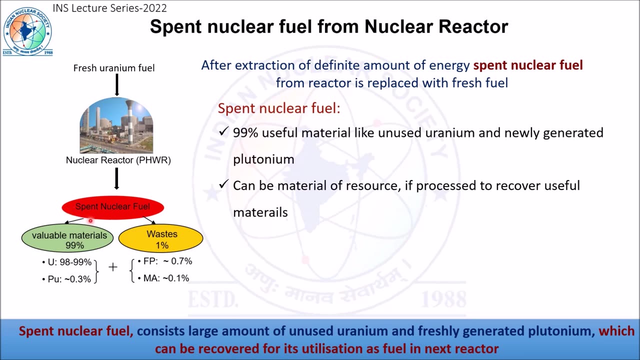 by the nuclear reactor. Only 1% of uranium is getting consumed inside the nuclear reactor. So if we examine the overall constituents of the spanned nuclear fuel, we can see that the 99% of the material of the spanned nuclear fuel is either unutilized uranium or freshly. 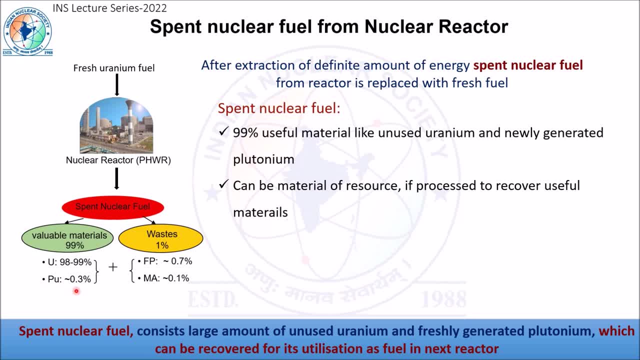 generated plutonium, both of which has potential as the fuel in the nuclear reactor, And only 1% of the material of the spanned nuclear fuel can be consumed by the nuclear reactor. So we can see that the spanned nuclear fuel can be considered as a waste, which mainly 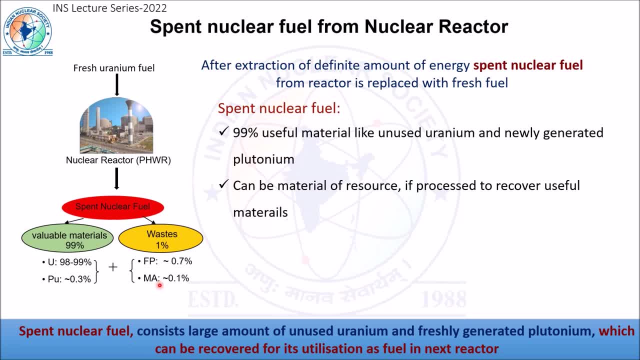 consists fission product and minor actinide. However, in our subsequent lecture we will see that some of the fission product and minor actinides have also have useful application in societal applications and they can be recovered for those applications. then waste volume can be further reduced. 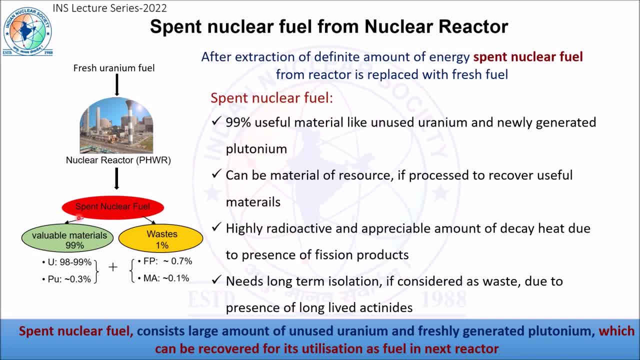 The spanned nuclear fuel immediately coming out from the nuclear reactor contains high amount of radium. This means that the spanned nuclear fuel can be stored in a water-cooled pool for safe removal of decay heat and providing adequate shielding for high amount of the radioactivity. 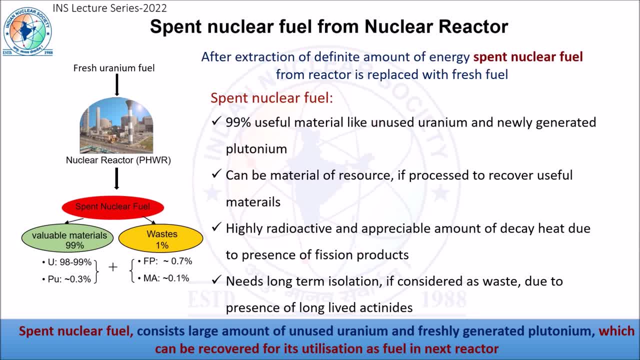 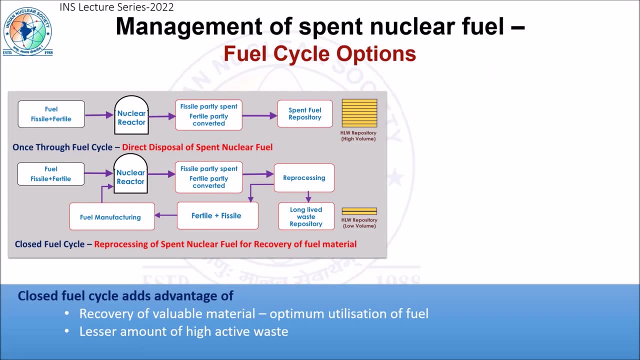 After ensuring the cooling of the spanned nuclear fuel for certain number of years, the spanned fuel are taken up for the safe management. Now let us see what are the strategy for management of this spanned nuclear fuel. Two major fuel cycle options are being implemented for safe management of spanned nuclear fuel. 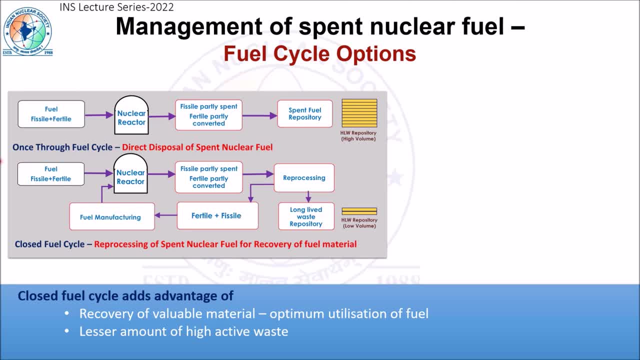 In the first fuel cycle option, which is based on one's through fuel cycle, where the spanned nuclear fuel coming out from the reactor is considered as a waste and is not aimed to process for recovery of unutilised uranium and plutonium present in the spanned nuclear. 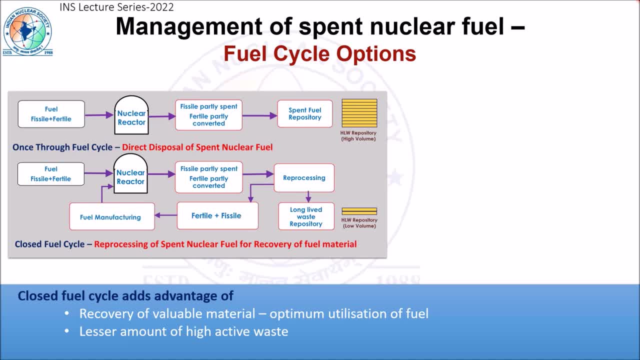 fuel. However, this spanned nuclear fuel will be released. The spanned nuclear fuel will be released in the nuclear reactor in 3 days and the primary Interimly stored for certain amount of years, and then they will be safely disposed in deep geological repository. 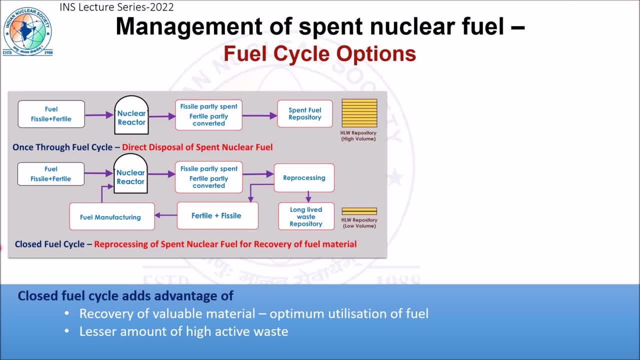 While in second fuel cycle option, which is based on the closed fuel cycle, where the span nuclear will coming out from the reactor is considered as a material of resource and is aimed to process for recovery of unutilized uranium and plutonium present in span nuclear fuel. 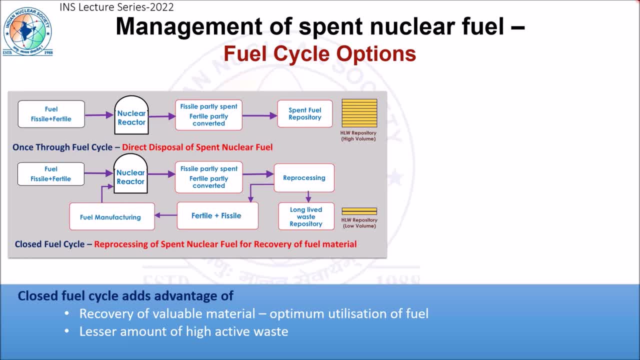 Thus recovered uranium and plutonium will be utilized as a fuel in next. So in case of closed fuel cycle, where the unutilized uranium and plutonium is are recovered for their utilization in a nuclear reactor for production of the energy and electricity, closed fuel cycle gives advantage of 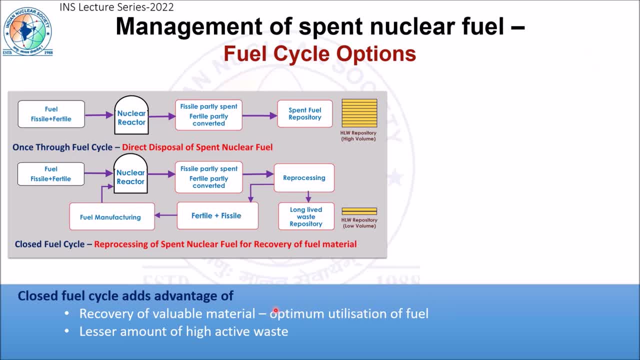 optimal utilization of a fuel. if we take a case of PHWR, where we have seen that the span- 99% of the constituent of span nuclear fuel- are unutilized uranium and plutonium and in closed fuel cycle this uranium and plutonium are recovered for their utilization as a fuel in next reactor. as a result, 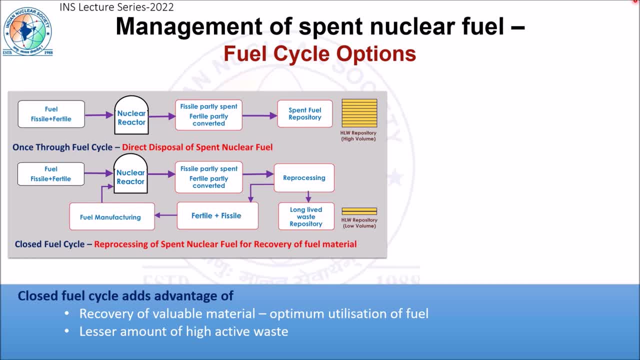 The closed fuel cycle not only give the advantage of optimal utilization of fuel, but it also helps in generation of the lesser amount of the high active waste, because the major portion of span nuclear fuel, which is Uranium and plutonium, are being recovered for their utilization as a fuel in next reactor. 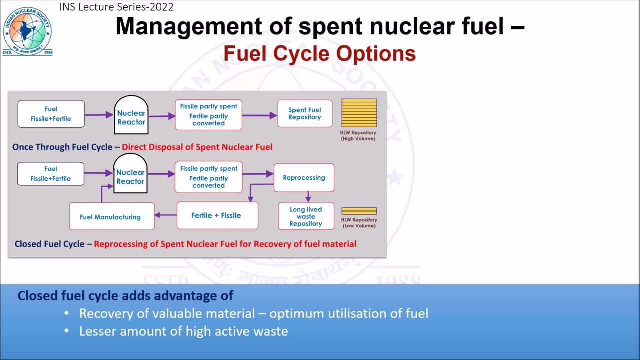 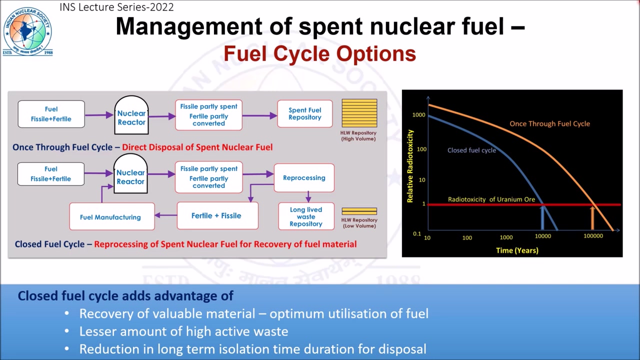 Earlier. the radiotoxicity of nuclear waste reduces with the time and we need to isolate the nuclear waste for certain time duration So that it's a radiotoxicity reduces to the safe level and It will not be further harmful. closed fuel cycle adds another Advantage that the time duration required for long-term isolation of high active waste which we need to dispose in deep geological repository. 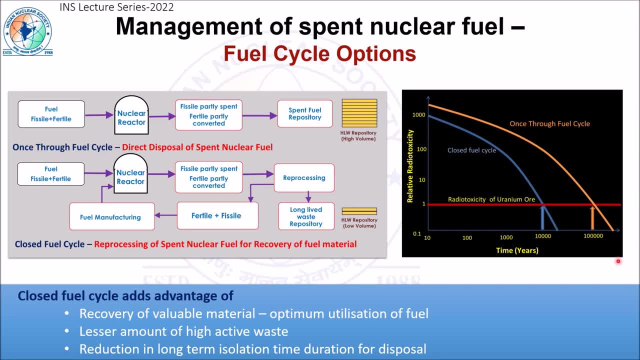 reduces significantly in case of the closed fuel cycle as compared to the once through fuel cycle. Remember, in once through fuel cycle We need to dispose span nuclear fuel, as it is in deep geological repository, while in closed fuel cycle we recovered the uranium and plutonium and the only 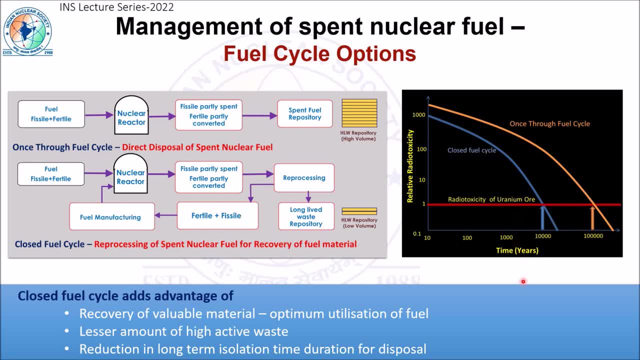 Remaining fission products and minor actinide will be disposed as a high active waste in deep geological repository. Here we have considered the same level of radiotoxicity as equivalent to the radiotoxicity of uranium ore, because we know that the uranium ore are naturally available and 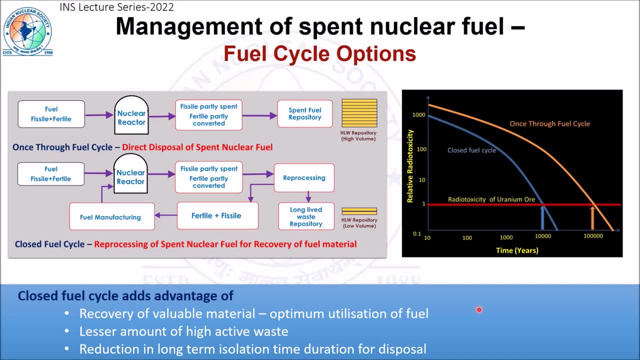 It has not adversely harmed the ecosystem. as a result, the closed fuel cycle gives three major advantages: that it helps us in optimal utilization of fuel, It reduces the final waste volume of high active waste and it also Reduces the time duration required for long-term isolation of high active waste during disposal. 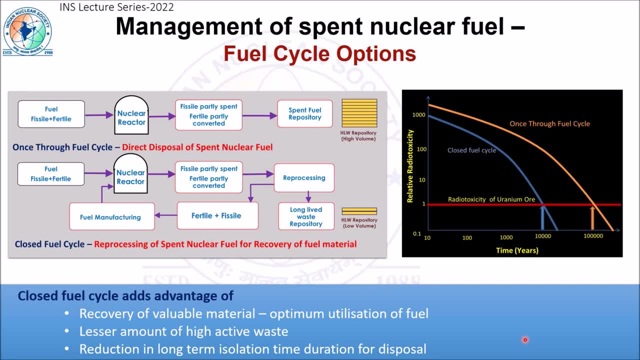 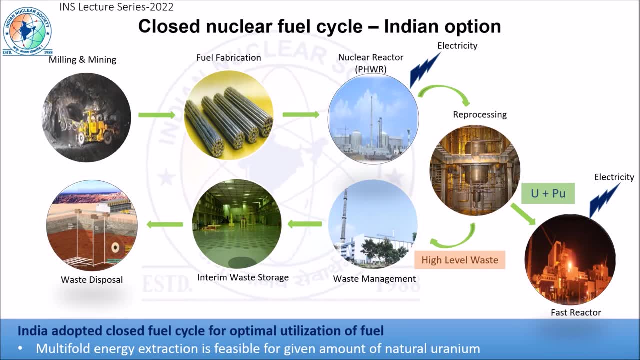 besides this, the closed fuel cycle also opens up an Opportunity to recover the valuable radionuclide for their societal application. between the advantages of closed nuclear fuel cycle option, India has adopted the concept of closed nuclear fuel cycle option for management of span nuclear fuel. The concept has already been put in practice for management of span nuclear fuel arising from various PHWRs. 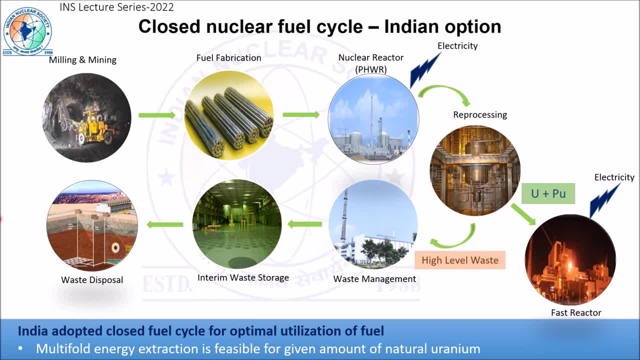 Which are under operation for generation of electricity using nuclear energy in our country. If we take a case of closed nuclear fuel cycle of PHWR, The first of all uranium is getting mined and milled From uranium ore, and thus extracted uranium is further Converted into the uranium oxide form. this uranium oxide is further converted into the small cylindrical pellet form. 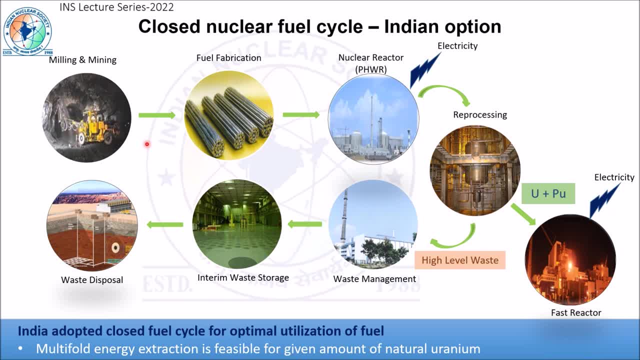 Which will be put inside the zircolite tube to make a fuel pin. such 19 fuel pins are put together to make a cluster of fuel bundle, and Then this fuel bundle will be put inside the nuclear reactor. and in case of- in our case- This is not an issue. 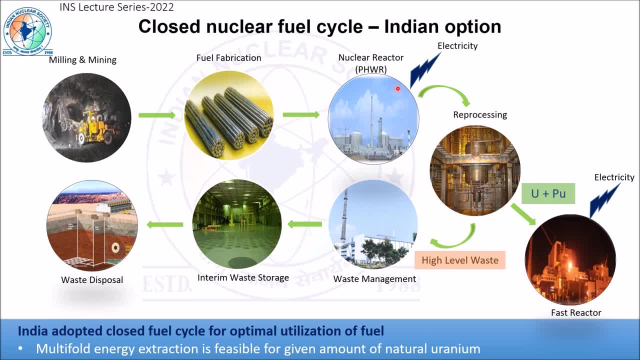 But we can get back to the historical business of하다. we will come back to it later. Now, here we come back to a simple example of a huge plant that is coming out from a nuclear reactor. we need to transfer the oxygen from the reactor to somewhere in the upper region of the nucleus, to an organic cell pool. and then we have to take this carbon dioxide into the nuclear reactor, and that is a very important factor for the generation of hydrogen and electricity. after extracting the definite amount of energy from the fuel, the fuel has to be replaced with the fresh fuel, and the span fuel coming out from the reactor is having considerable good amount of the radioactivity as well as decay, and hence they need to store inside the water cooled pool for certain amount of years and therefore you have to measure the energy and the amount of oxygen that is stored in the reactor after you have taken it into the reactor. 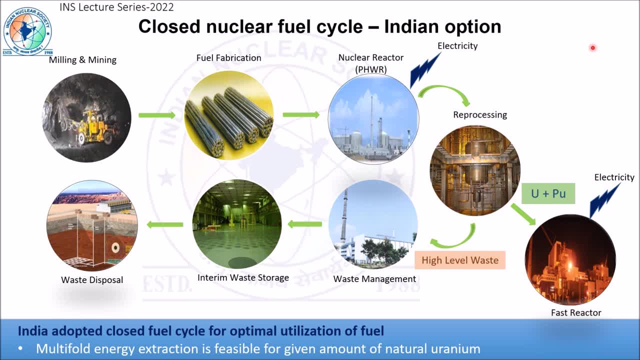 the cooling of spent nuclear fuel inside the water-cooled pool for about three to five years. the spent nuclear fuel can be subjected to the complex radiochemical process for extraction of uranium and plutonium, and this complex chemical process is called reprocessing While reprocessing. 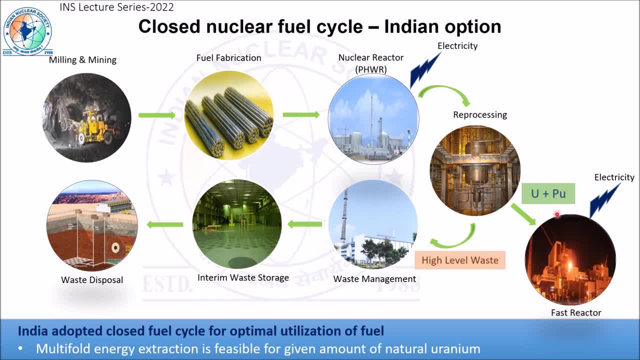 the spent nuclear fuel, the uranium and plutonium can be separated, which can be further converted into the fuel for their utilization in a fast reactor program for production of the electricity. In our country the fast reactor has been considered as a second stage of our nuclear power program. The remaining fission products in minor actinides of spent. 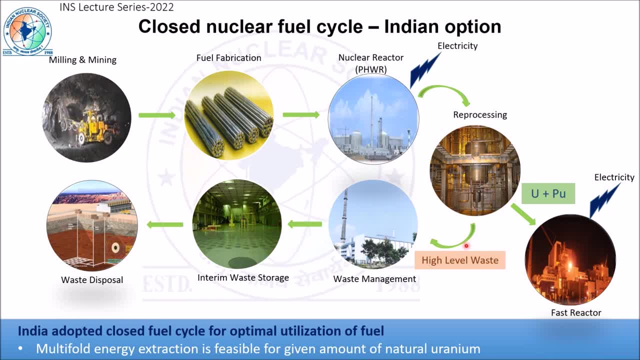 nuclear fuel will come out as a high-level waste from the reprocessing, and this high-level waste will be further concentrated and contained or immobilized in inert glass matrix. Thus immobilized high-level waste in glass matrix will be further interimly stored in air-cooled water for 25 to 30 years, and then they will be finally subjected to the disposal in. 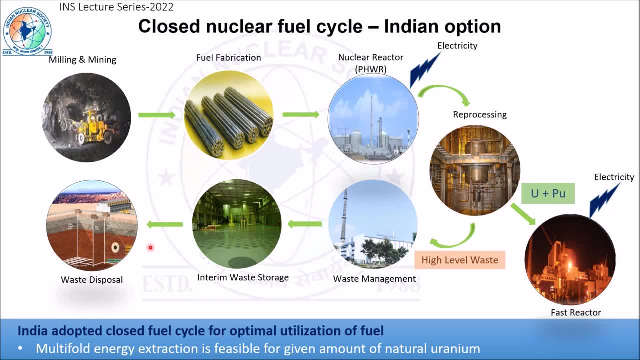 deep geological repository as a high active waste. With the advent of the new technology, the valuable radionuclides present in high-level waste are also aimed to recover for their potential applications in various societal applications. In our subsequent lecture we will see that how this uranium and plutonium is getting extracted from the spent nuclear fuel. 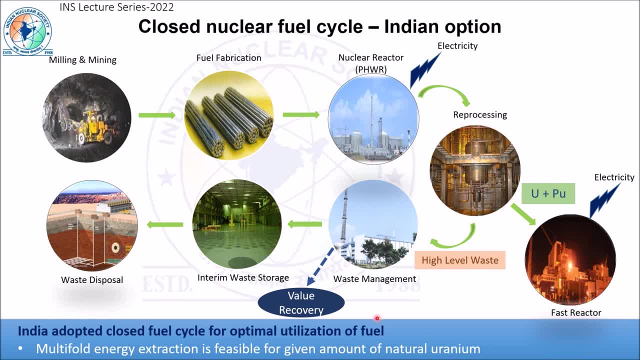 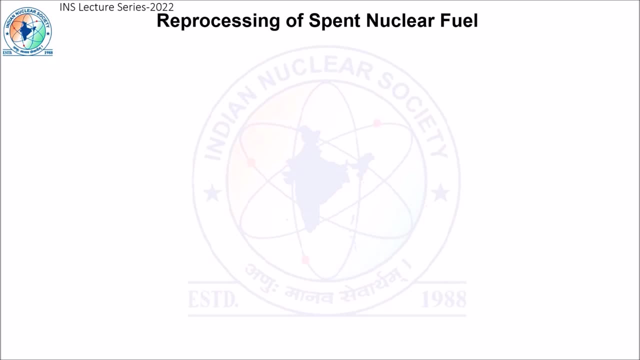 by the process called reprocessing, and how do we manage the high-level waste, along with the recovery of valuable material for societal application? Now let us see how the spent fuel are reprocessed. after ensuring adequate cooling of spent fuel for about three to five years, they are subjected to the reprocessing. 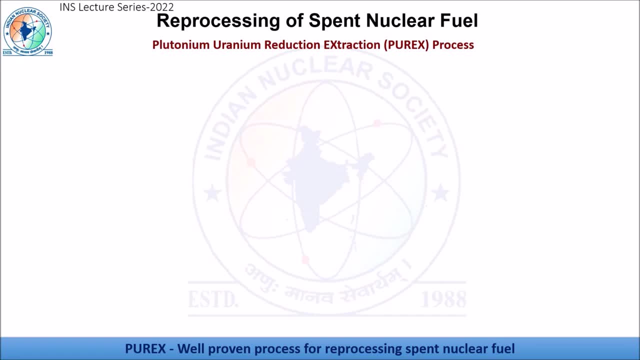 A well-proven solvent structure-based purex process has been successfully deployed for reprocessing of spent fuel arising from PHWRs. As a first part, the spent fuel are chopped into the small pieces, and then these small pieces are put into the boiling nitric acid to dissolve the fuel material. 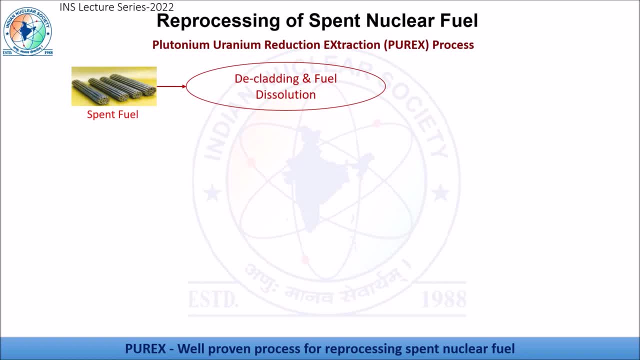 The boiling nitric acid dissolves the fuel material, including uranium, plutonium, fission product and minor actinide, leaving behind the zircolite tube undissolved. Thus generated dissolved solution mainly containing uranium, plutonium, fission product and minor actinide is further subjected to the 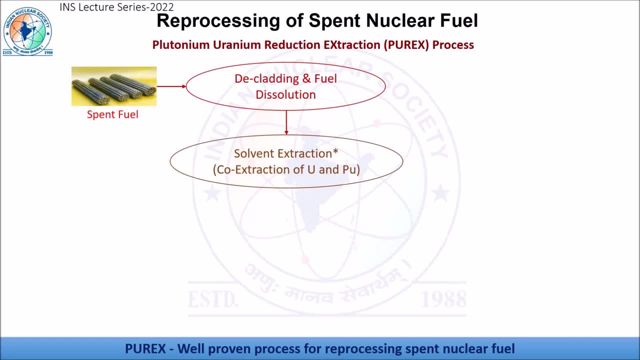 solvent extraction process for extraction of uranium and plutonium, leaving behind an aqueous stream which mainly contains fission product and minor actinide. This aqueous stream, which contains mainly fission product and minor actinide, is further concentrated using evaporation process. 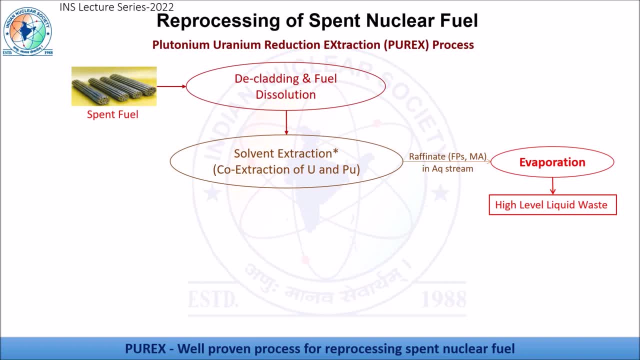 to convert it into the high-level liquid waste. The extracted uranium and plutonium is further subjected to the partitioning process to separate out the uranium and plutonium from each other in nitrate form. Thus separated uranium nitrate and plutonium nitrate are further subjected to the 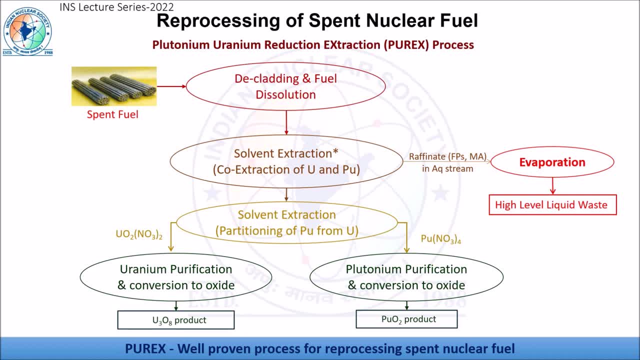 purification step separately, and then purified uranium nitrate and purified plutonium nitrate is further converted into the oxide separately. Thus generated uranium oxide and plutonium oxide in very purified form can be used as a fuel in fast reactor program. In India we have more than 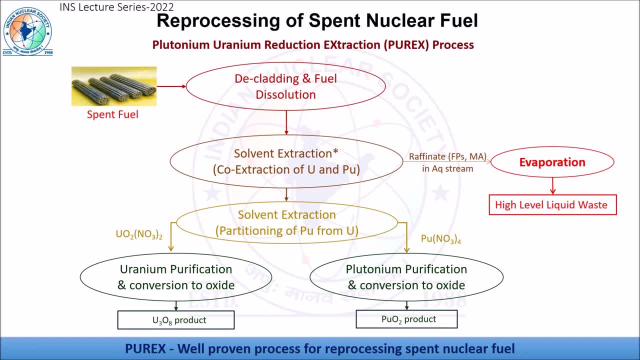 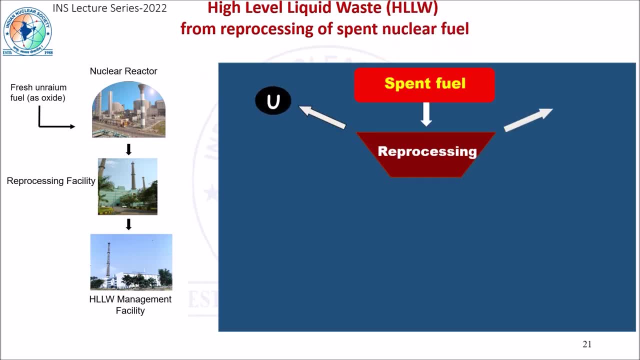 six decades of experience for safe refueling of uranium nitrate and plutonium nitrate. After recovering the uranium and plutonium by reprocessing of spent fuel, a high-level liquid waste is getting generated which mainly contains fission products and minor actinide, which were 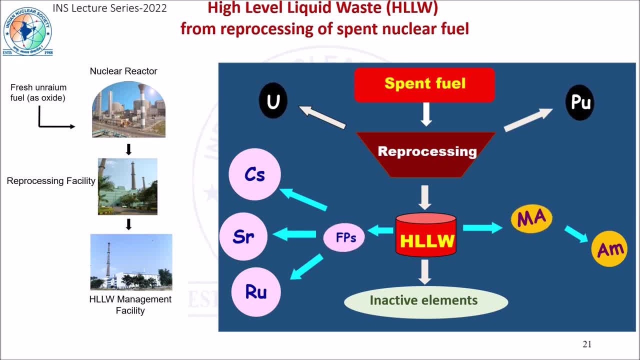 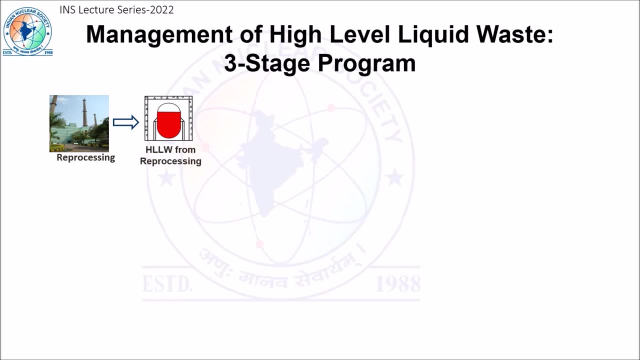 earlier present in spent fuel, as well as inactive elements which have been added during the reprocessing of a spent fuel. Now let us see how the uranium nitrate and plutonium nitrate are getting managed, As the high-level liquid waste contains appreciable amount of radioactivity. 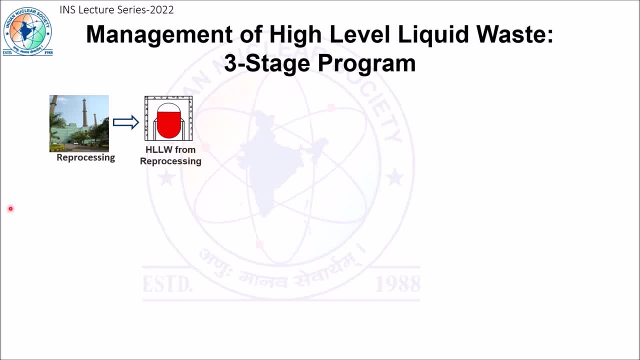 either due to fission product or minor actinide, and also contains considerable amount of decay heat, a special attention needs to be given while their management. The long-term storage of high-level waste in liquid form is certainly not desirable, because the chances of migration of radionuclide will be considerably higher if we store the. 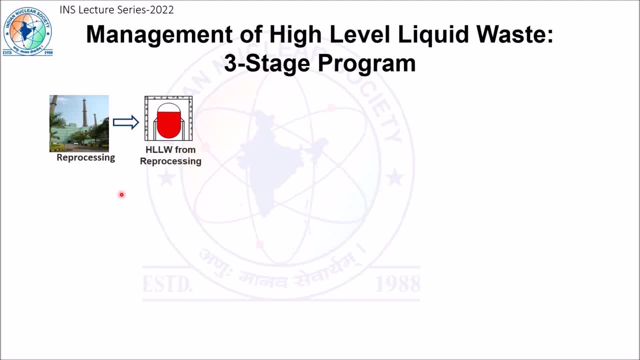 high-level waste in liquid form for longer duration. As a result, a three-stage program have been developed, demonstrated and successfully deployed for safe management of high-level liquid waste. In first stage, the high-level liquid waste is converted into an inert glass matrix. 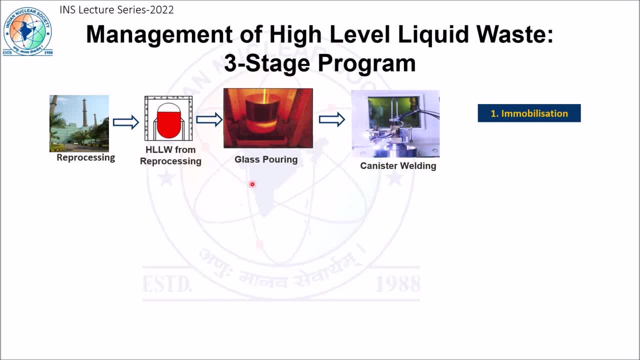 by a process called vitrification. By converting the high-level liquid waste into a glass matrix, we are aiming to immobilize the radionuclide of high-level waste in a glass structure, so that the migration of radionuclide to the environment can be eliminated. 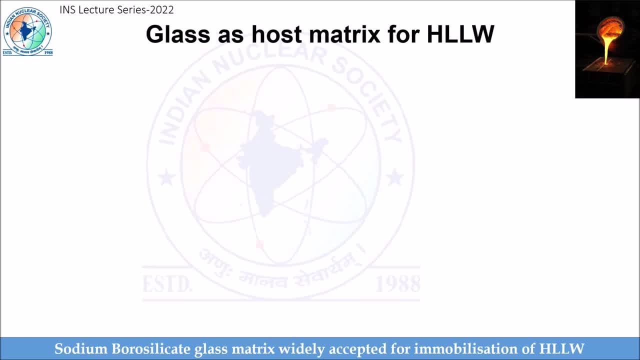 But the question arises why we have selected glass as a host, matrix or immobilization of radionuclide, which are present in high-level liquid waste, And the most important reason is its inert nature. Due to its inert nature, glass do not 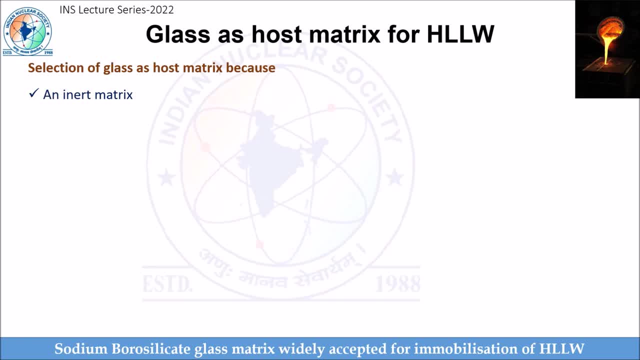 react very easily with any system. When we immobilize the high-level liquid waste into the glass matrix, the radionuclide of high-level liquid waste becomes part and partial of a glass molecular structure. As a result, the chances of leaking out of this radionuclide from glass matrix is almost negligible, and so the 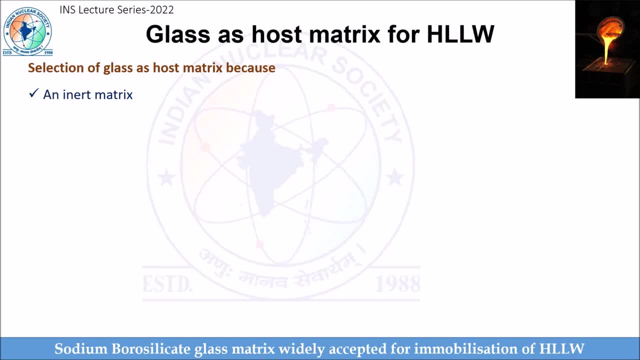 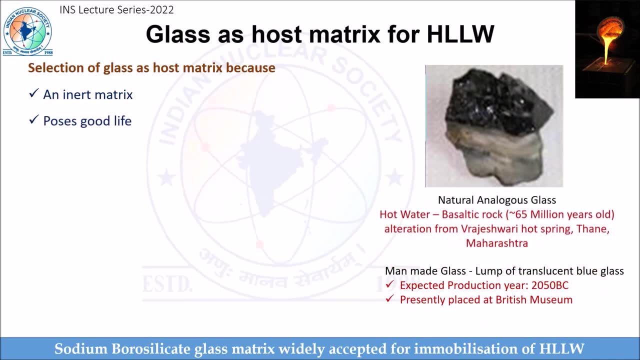 migration of radionuclide from glass matrix is almost negligible. Besides this, the glass also possess good life. The high-level liquid waste contains many radionuclide, which has considerably longer half-life, and so, whatever the matrix we do select, it should have considerably good life. There are many. 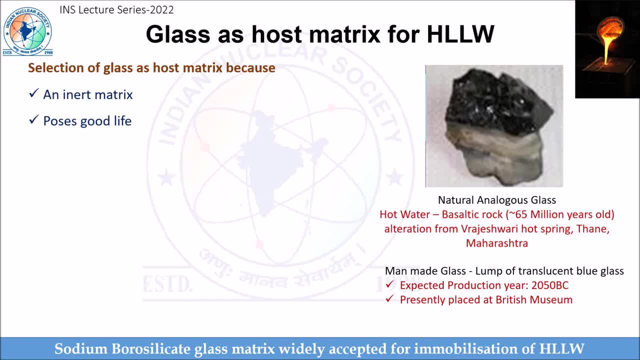 examples of either naturally origin glass or man-made glass which have shown considerably good life. So it gives us confidence that glass has a good life, which is a desirable condition for the host matrix. Besides this, the high-level liquid waste contains about 30 to 40 elements of periodic table. 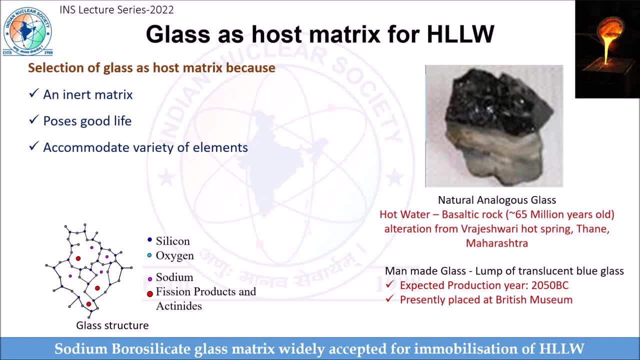 So the high-level liquid waste contains about 30 to 40 elements of periodic table. So the high-level liquid waste contains about 30 to 40 elements of periodic table And whatever the matrix we do select, it should have capability to accommodate these elements. The glass can accommodate variety of elements. The glass has very 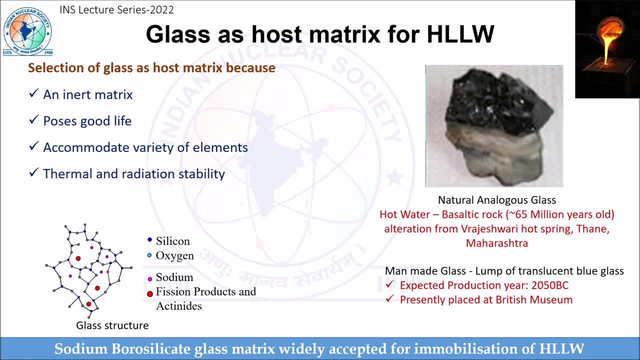 good thermal and radiation stability, which is also a desirable criteria for selecting a host matrix for immobilization of radionuclide of high-level liquid waste, And when we convert or immobilize the radionuclide of high-level liquid waste into the glass matrix, the overall waste. 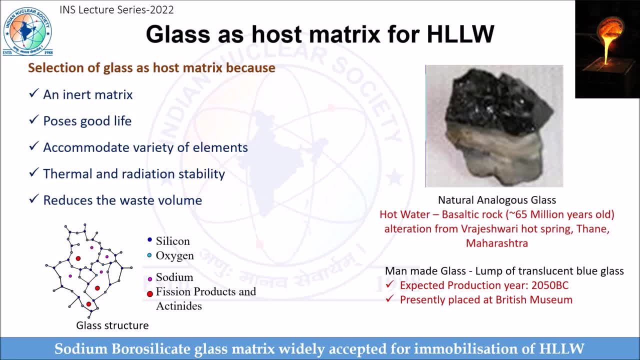 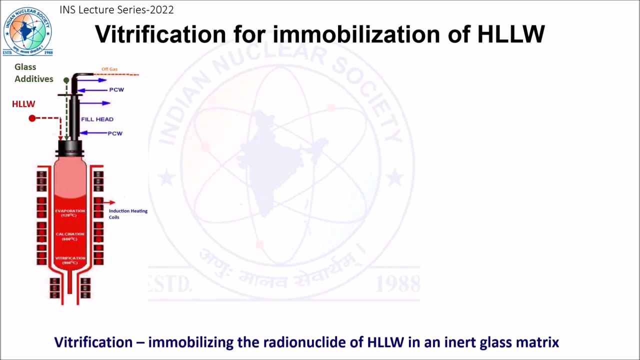 volume is reduced. Considering all these reasons, which are being offered by the glass matrix, the glass has been selected as a host matrix for immobilization of radionuclide which are present in high-level liquid waste. For immobilization of high-level liquid waste in glass matrix using vitrificol. 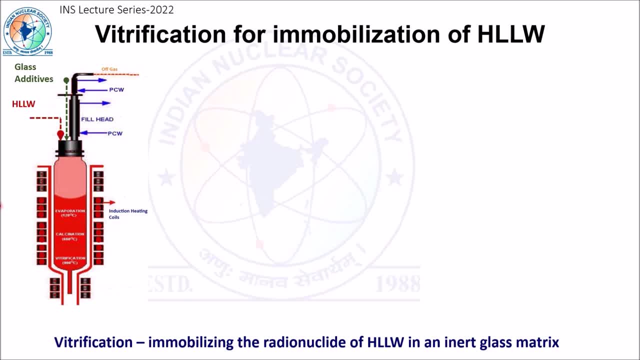 vitrification process, the definite amount of high-level liquid waste, along with glass making additives, are added into a special equipment called a melter. Then the melter is heated up to 950 degrees Celsius, by which various radiochemical processes are taking place inside a melter, which finally result in immobilization of radionuclide of high-level. 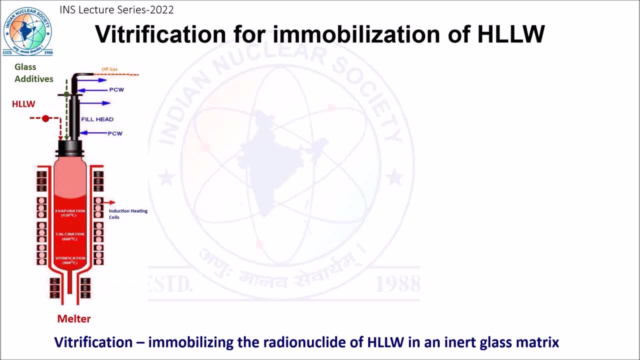 liquid waste into a glass matrix. Vitrification process poses many challenges, including associated high amount of radioactivity due to presence of high-level liquid waste, need of high operating temperature for making glass and presence of corrosive environment. All these challenges necessitates the special 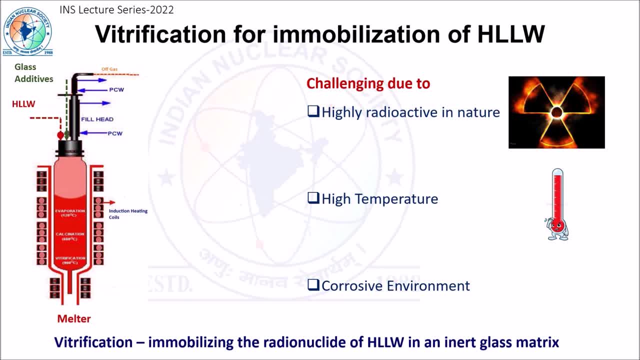 attention for design and development of melter technology inside which the complete vitrification process occurs. Besides this, the melter technology required for vitrification process needs to be placed inside the heavily shielded hot-cell area and needs to be designed with remote operation. 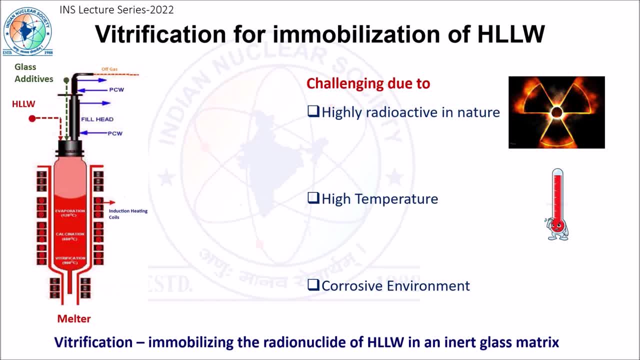 and remote maintenance provision so that the high amount of radioactivity can be handled very safely. Combining all these challenges makes vitrification technology and process more cumbersome. as a result, very few countries in the world could develop the vitrification technology successfully. China has developed, demonstrated and successfully deployed the vitrification technology at engineering. 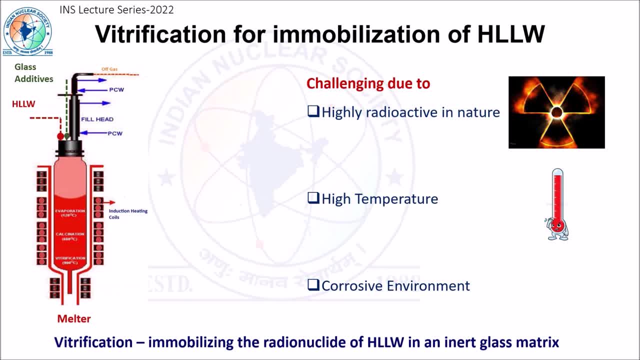 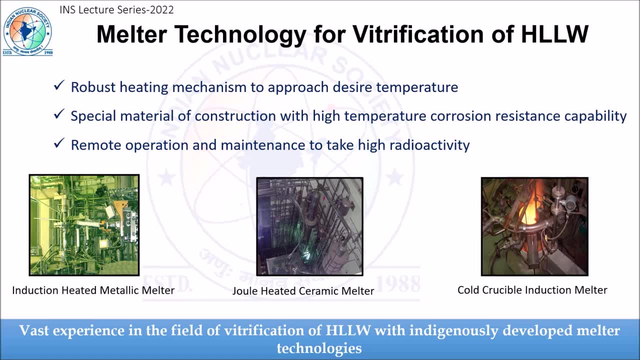 scale for immobilization of radionuclide of high-level liquid waste in a glass matrix. Development of melter technology for vitrification of high-level liquid waste is a very important task for vitrification of high-level liquid waste. While developing the melter technology, 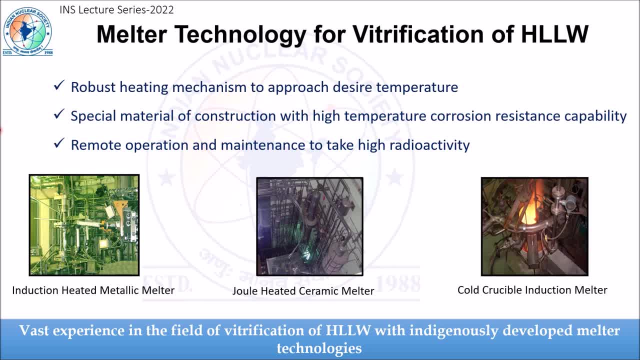 due care needs to be taken so that the treatment of the liquid waste can be performed in a high-level way. The challenges associated with high-level liquid waste can be overcome. As a result, in India, three different melter technologies have been developed successfully. 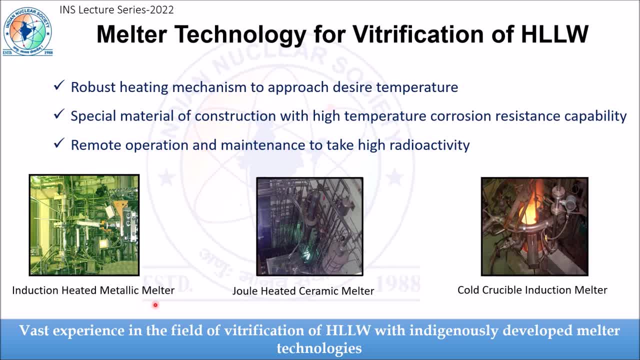 Out of which the induction-heated metallic melter and dual-heated ceramic melter have been successfully demonstrated and deployed for vitrification of high-level liquid waste, While cold-producible induction melter has been developed and demonstrated at inactive scale and will be deployed for vitrification of high-level liquid waste While cold-producible. 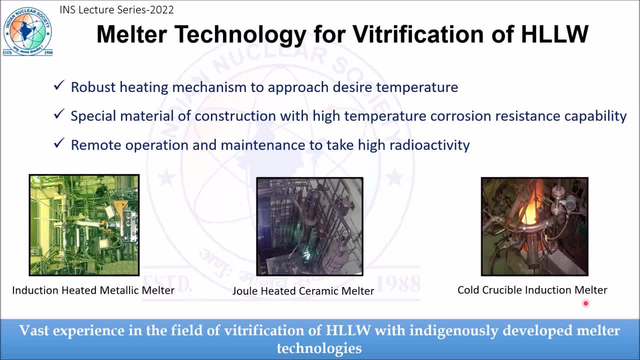 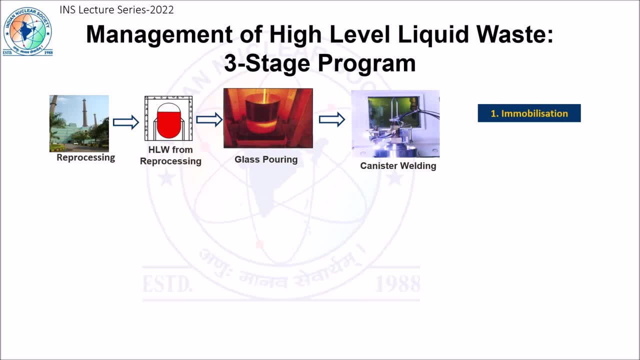 induction melter has been developed and demonstrated at inactive scale and will be deployed for vitrification of high-level liquid waste. After immobilizing the radionuclide of high-level liquid waste into a glass matrix using vitrification process, the molten glass containing vitrified high-level waste is then drained into the 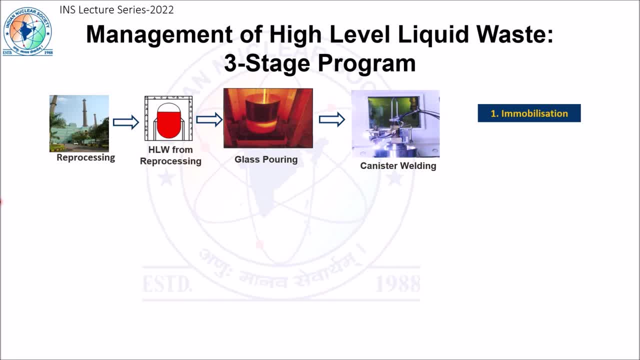 stainless steel container. This stainless steel container is then closed with a lid and remotely sealed using remote welding techniques. Thus generated stainless steel container containing vitrified high-level liquid waste is then drained into the stainless steel container level waste is then transported to an air-cooled storage vault where this vitrified high level 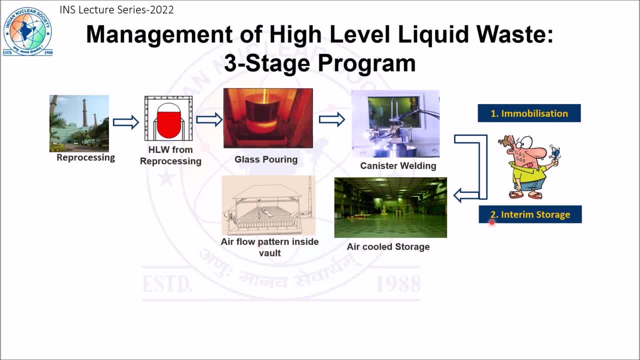 waste is intimately stored for safe removal of initial decay heat. These air-cooled vaults are designed in such a way that the natural draft of air removes the decay heat thus generated from vitrified high level waste, so that there will not be any accumulation of heat inside the stainless steel container containing vitrified high 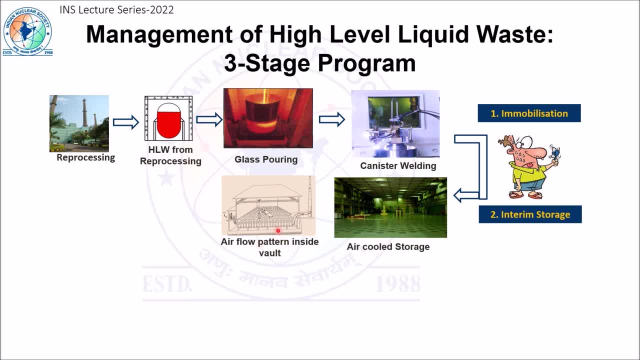 level waste and the temperature of same can be maintained well within the limit. In India, such two air-cooled vault interim storage facilities are under operation for interim storage of stainless steel container containing vitrified high level waste for safe removal of initial decay heat. 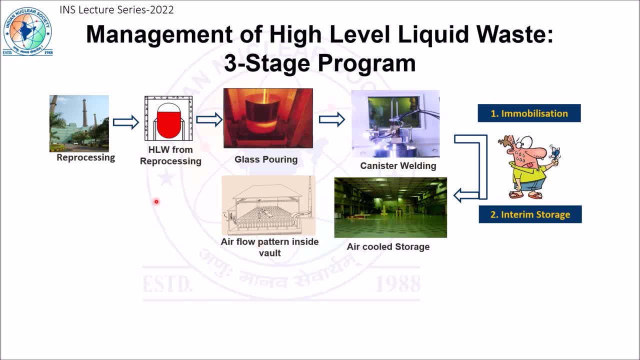 After ensuring that the air-cooled vaults are properly stored. the air-cooled vaults are then transported to an air-cooled storage facility After ensuring the interim storage for at least 25 to 30 years. this stainless steel container containing vitrified high level waste is then planned to be disposed in deep. 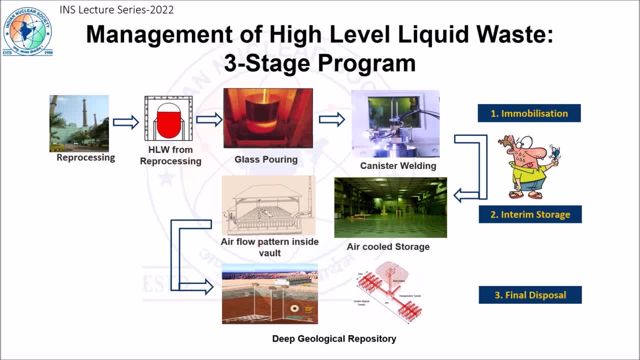 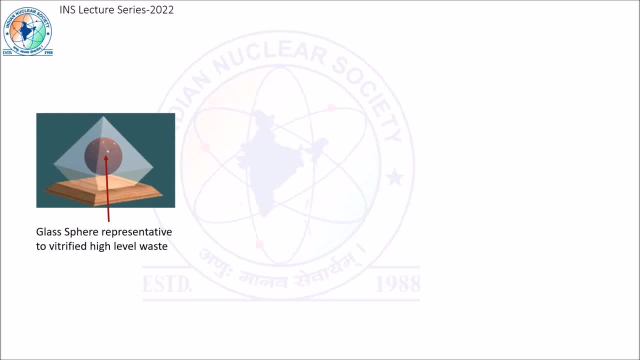 geological repository as a final disposal. We have already discussed that nuclear energy generates lesser amount of waste volume. That can further be illustrated by an example of high active waste getting generated from the closed nuclear fuel sites fuel cycle. for example, if we take an indian nuclear family consisting a member of four, 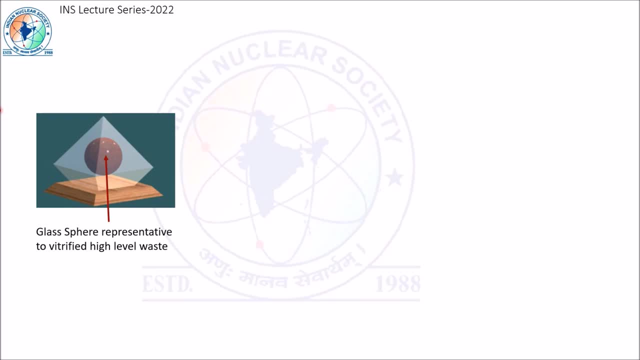 taking their old need of electricity using nuclear energy for entire life. here the life expectancy we have taken as a 60 years. then the amount of high active waste getting generated following the closed fuel cycle is only a small sphere of 40 mm dia. such a low amount of the waste is getting. 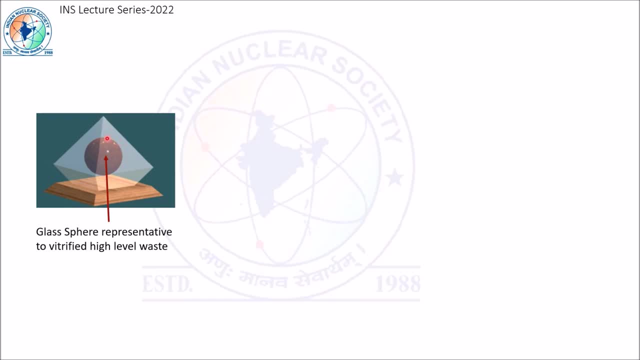 generated from close nuclear fuel cycle. but we need to think further that can we further reduce the waste? can we earn the wealth from the nuclear waste? and this type of food for thought gives us further trigger for the development of nuclear waste management for for safe and efficient. 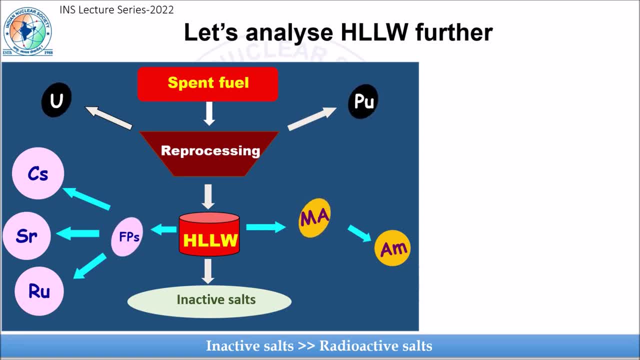 management. now let us analyze the high level liquid waste further. we have seen that the spent fuel reprocessing generates the high level liquid waste, which contains fission products and minor actinides, which are the major contributor towards the radioactivity of high level liquid waste. besides this high level liquid waste also contains inactive salts or inactive constituents. this 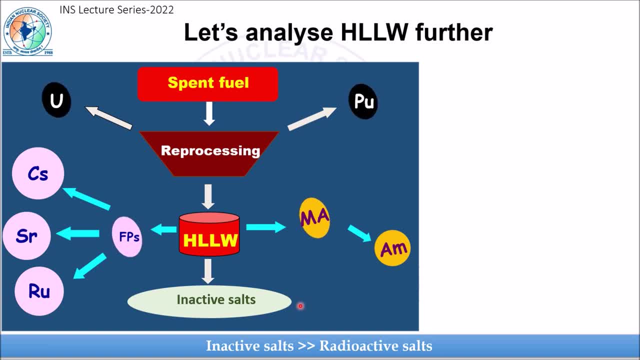 inactive constituents do not contribute to the high level liquid waste but they contribute to much in a radioactivity of high level liquid waste but they do presence in much larger quantity as in as comparison to the fission product and minor actinide. if we analyze the overall 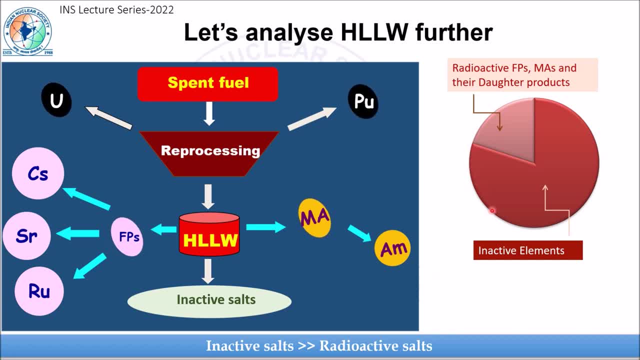 composition of high level liquid waste. we can see that this- inactive elements or inactive constituents- makes the major fraction of the high level liquid waste, as compared to the radionuclide, which are either formed in form of fission products and minor actinide. we need to develop 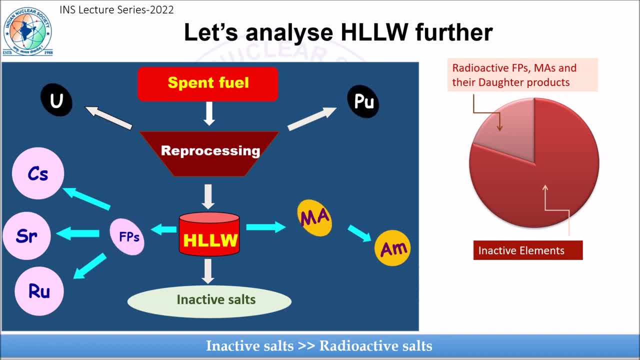 the technology of fission products and minor actinide. we need to develop the technology of fission products and minor actinide. we need to develop the technology of by which we can separate this radionuclide from the inactive elements and we can treat this radionuclide separately. 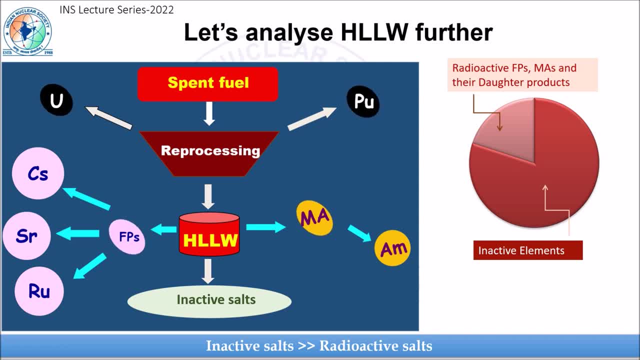 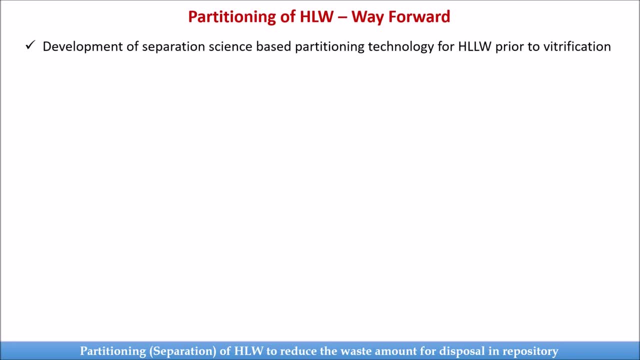 so that the final waste volume can be minimized drastically. for the same separation, science-based partitioning technology has been developed for separation of these regular radionuclides from high level liquid waste. utilizing this technology, radionuclides, including high level liquid waste, including fission product and minor actinide, can be partitioned or separated from high level liquid. 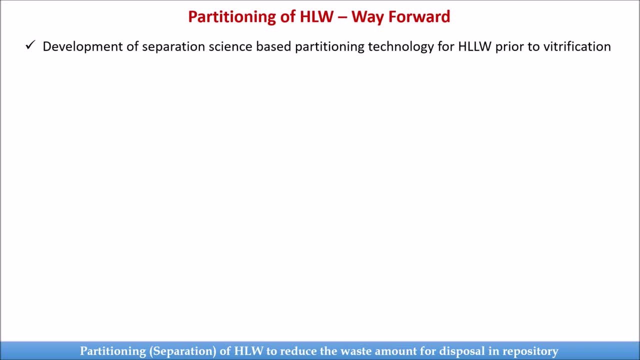 waste and then that they can be subjected to treatment or vitrification in glass matrix separately, so that the final vitrified waste volume can be reduced. with the advent of this technology, even selective separation of radionuclide is also feasible. for example, we know 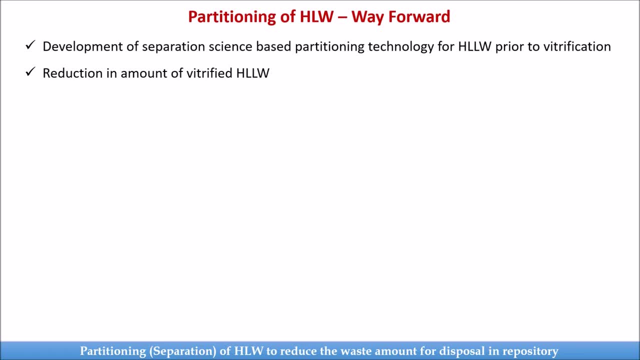 that high level liquid waste contains minor actinides, and these minor actinides are having considerable longer half-life and they decay with the series of alpha particle as well as beta gamma radioactivity. it is these minor actinides which are mainly responsible for long-term concern of high level 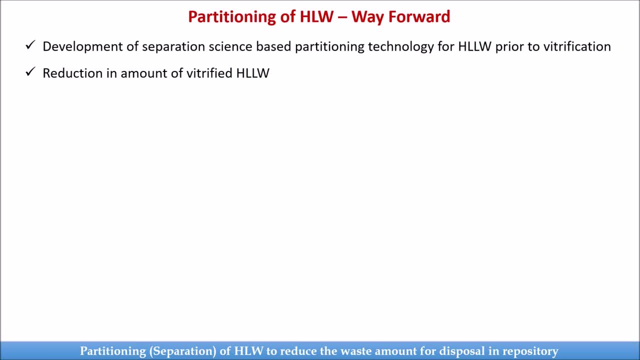 liquid waste. utilizing the partitioning technology, the selective extraction of minor actinides, such as emerysham 241, can be done, and then this is selectively separated. minor actinide can be vitrified separately, separately, so that the final vitrified waste volume is reduced drastically. and it is this. 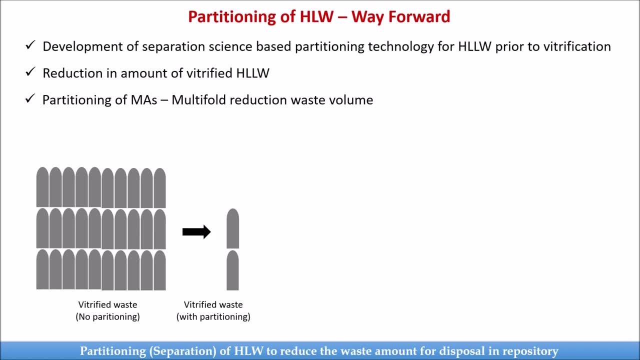 vitrified waste which contains the minor actinides, are required to be disposed in deep geological repository. as a result, by the partitioning of minor actinides and separately vitrification of these minor actinides, the final vitrified waste volume can be reduced by a multifold. 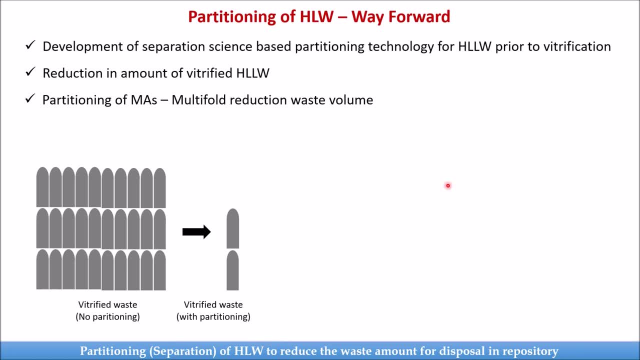 such as drastic reduction in vitrified waste, can help us in minimizing our need for final disposal in deep geological repository. besides this, this minor actinide can be fissioned in fast neutron spectrum if we separate the minor actinide or partition the minor actinide. 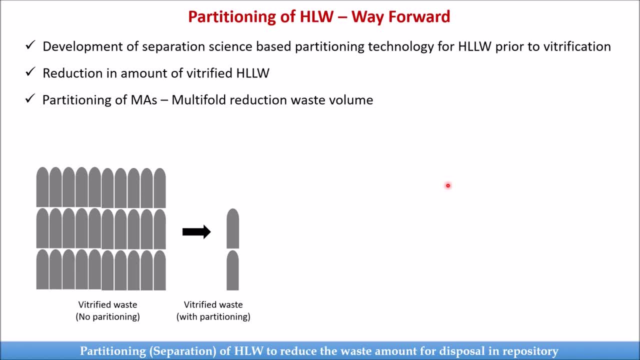 in purified form, this minor actinide can be converted into the fuel, and then they can be subjected to the fast reactor, where this minor actinide can be converted into the fuel and then they can be fissioned into the two smaller half-lived fission products. as a result, 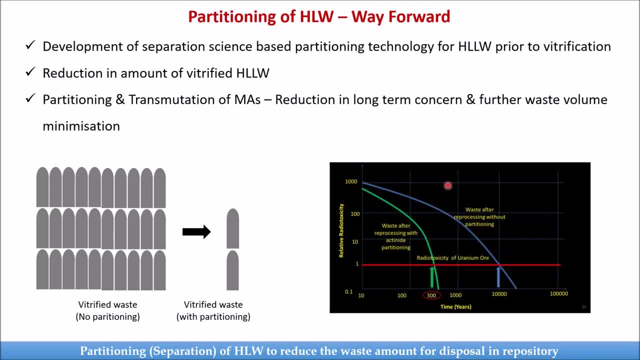 the partitioning, followed by transmutation of minor actinides in fast neutron spectrum can also help in reducing the long-term concern. the requirement of isolation of vitrified waste for the longer duration can be further reduced, And this is how The partitioning and transmutation of minor actinides helps us in reducing the long-term. 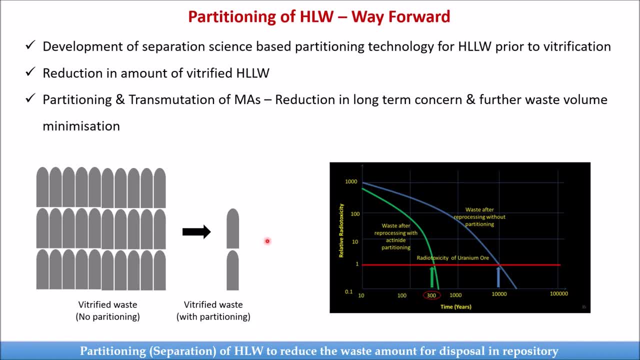 concern, as well as reducing the final vitrified waste with multifold amount. but for the same, the partitioning of minor actinide is a first step and most important step. besides this, the partitioning of high level waste also helps us in selective extraction of the radionuclide. 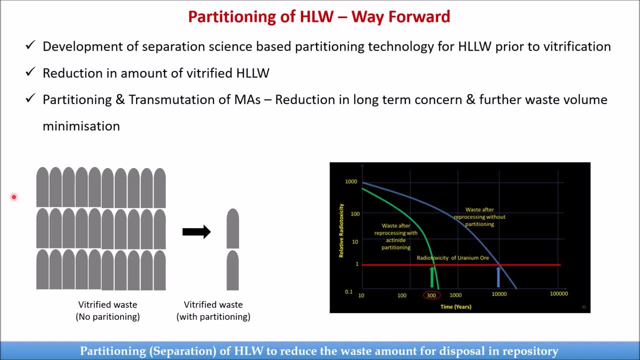 and some of these. radionuclide has various functions. So this is the first step. The partitioning of high level waste has various societal application. so, utilizing this partitioning technology, a recovery of valuable radionuclide from high level waste is feasible, which helps us in converting the nuclear waste into the wealth. 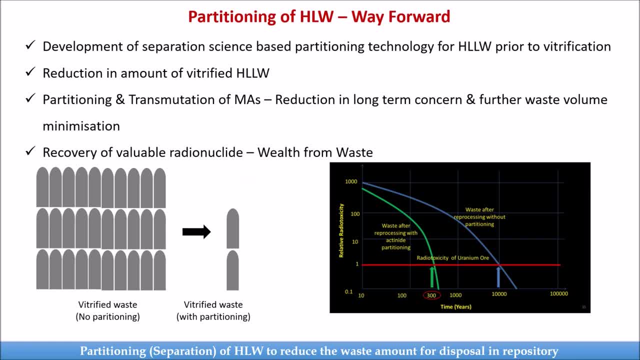 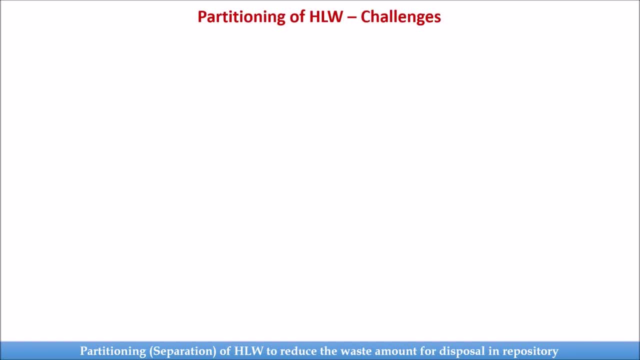 We will study this wealth from nuclear waste concept in detail in subsequent portion of the lecture. however, the partitioning of high level waste has few challenges which need to be overcome For getting success and advantages of this partitioning technology. the first and most important challenge is to develop the novel extractant, which should be capable to extract. 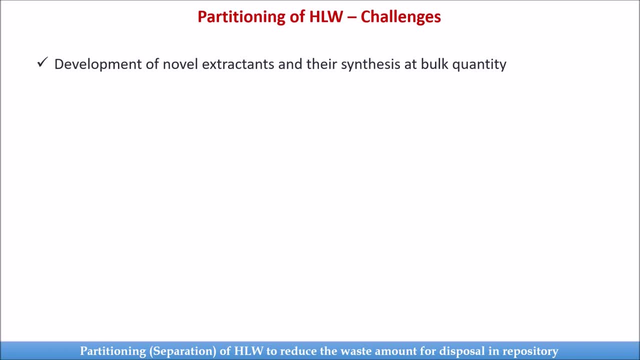 these radionuclide selectively from high level waste and then their synthesis at bulk quantity so that they can be utilized at engineering scale for treatment of bulk amount of high level waste. for separation of the radionuclide selectively. Based on this, we will discuss the following: 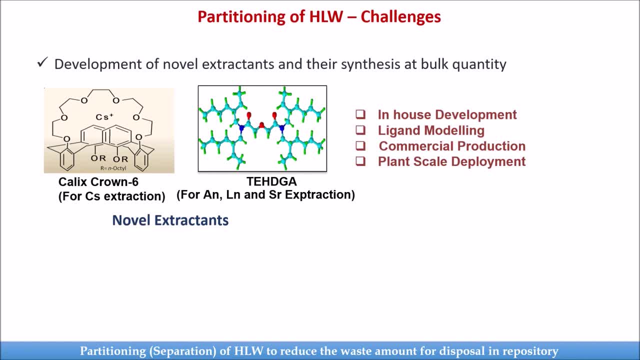 The first and most important challenge is to develop the novel extractant which should be capable to extract these radionuclide selectively from high level waste and then their synthesis at bulk amount of high level waste so that they can be utilized at engineering scale. sono theOhr- the interesting challenge, So now we are going to continue the same. 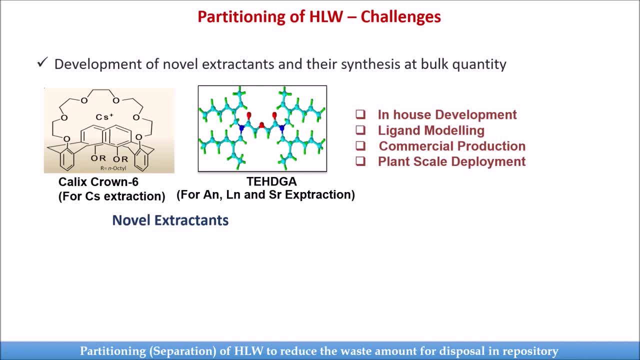 process. even some of the other points on partitioning technology are been developed which are capable of extracting the radionuclide from the high level waste and then same could be synthesized at bulk quantities so that they can be deployed at engineering scale 3.. 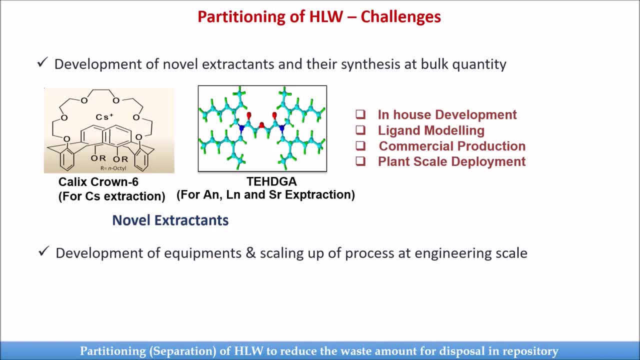 and scaling up the complete partitioning process at engineering scale. Due to continuous R&D efforts, the solvent extraction based process along with special contactors could be developed which can be utilized for partitioning technology, and same could be demonstrated at engineering scale for treatment of high level waste. 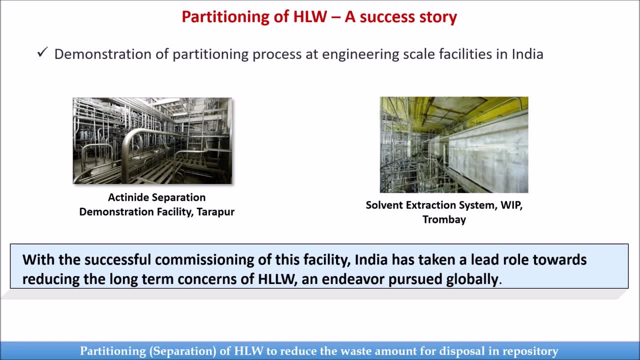 Based on the R&D efforts, the partitioning of high level waste could be successfully demonstrated. in India. There are two such facilities which are designed, constructed, commissioned and are under operation based on the solvent extraction based partitioning process for partitioning of high level waste. 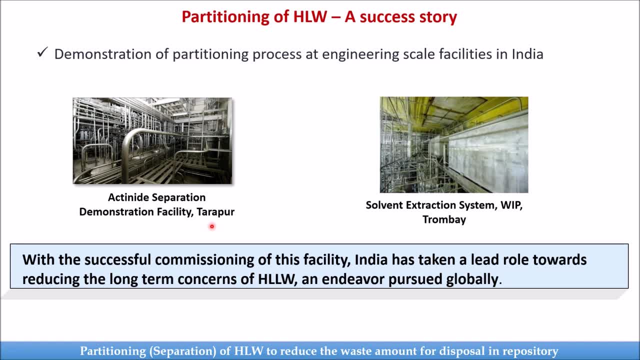 The first facility is at Tarapur, named actinide separation demonstration facility, where the partitioning of high level waste can be successfully demonstrated. The partitioning of minor actinide like Emrysium-241 could be successfully demonstrated from high level waste, While the second facility is at waste immobilization plant BARC Trombe, where the partitioning of 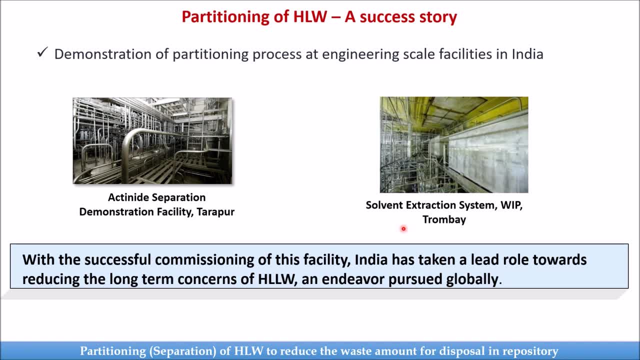 radioactive elements from inactive elements of HLW could be successfully demonstrated. Besides this, the selective extraction of valuable radionuclide like cesium-137,, strontium-90, and carotene-106 could also be demonstrated at this plant. 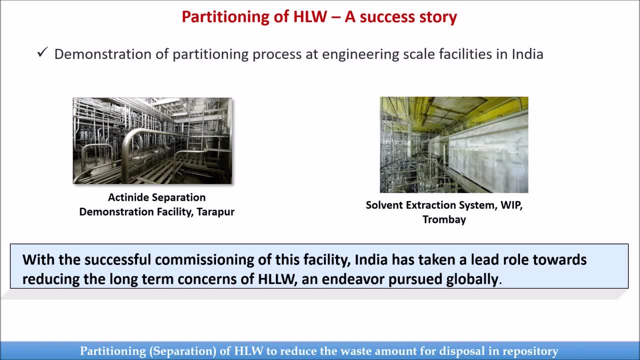 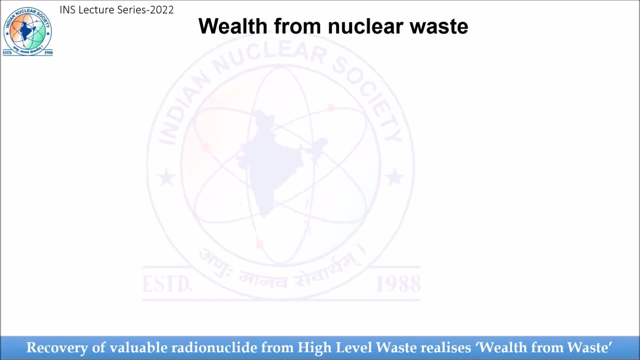 As a result, the partitioning of high level waste could be demonstrated, with the objective of overall reduction of the final vitrified waste volume, minimization of long-term concern, as well as value recovery for various societal applications. This partitioning technology can be used to reduce the value of waste. 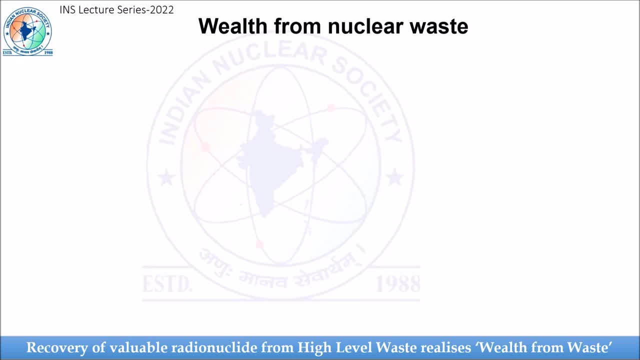 can also enable us to recover valuable radionuclides from high-level waste for their societal application. In high-level waste there are many fission products as well as minor actinides which have potential applications in various societal utilization. For example, cesium-137 is one of the prominent fission. 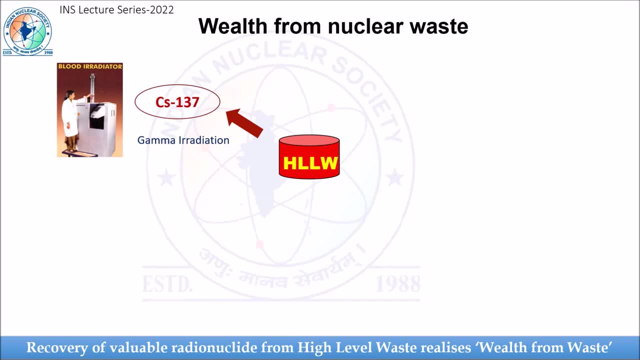 products in high-level waste which can be utilized for various gamma irradiation. Strontium-90 is another prominent fission products which can be utilized for the radiopharmaceutical application. Another fission product, ruthenium-106, which is present in high-level waste, can be recovered and can 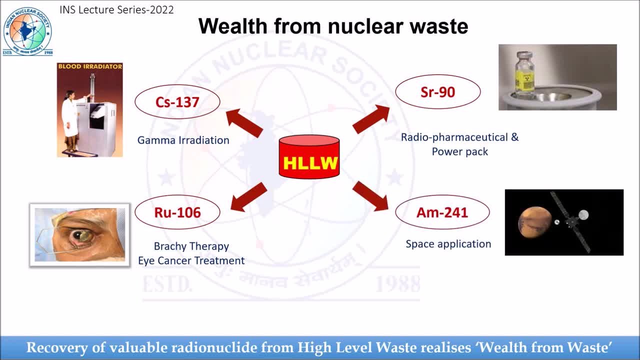 be utilized for eye cancer treatment, while the ambrosium-241, which is one of the prominent minor actinides present in high-level waste, can be recovered in purified form and can be utilized in various special application. So this valuable radionuclide can be extracted from high-level waste using partitioning. 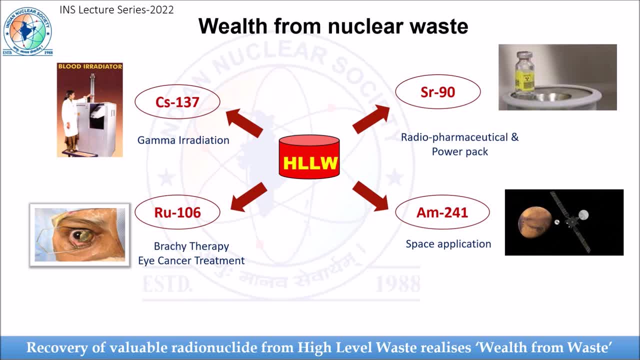 technology for various societal application. Utilizing of this radionuclide for societal application not only help us in reducing the waste burden, but also help us in realizing the concept of wealth from nuclear waste. Now let us see how this radionuclides are being extracted, recovered and being put. 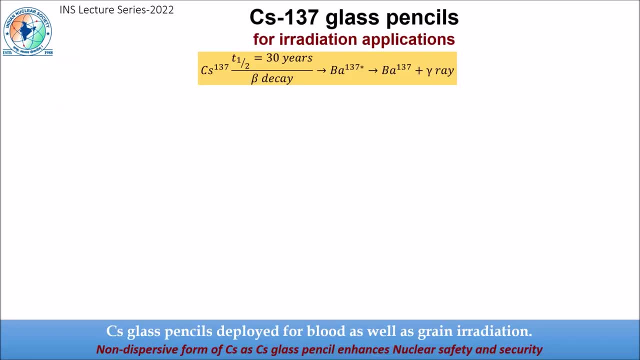 for societal application. We can see the prominent fission product present in high-level waste, cesium- 137.. The cesium-137 is radioactive in nature and decays to the barium-137 by emission of a beta particle. This barium-137 is at the excited state and 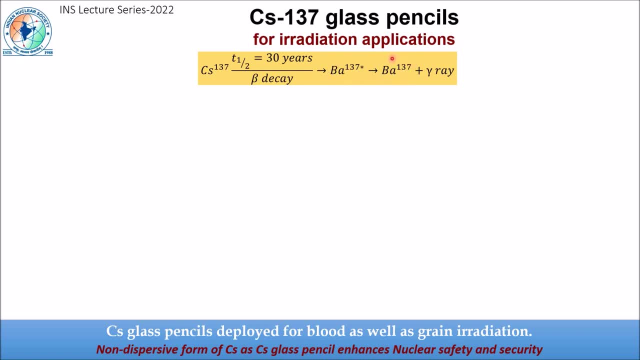 comes to the ground state as the stable barium-137 product by emission of a gamma ray. So the cesium-137 finally decays to the barium-137 by by emission of a beta particle and a gamma ray. The energy of this gamma ray is about 667 keV. 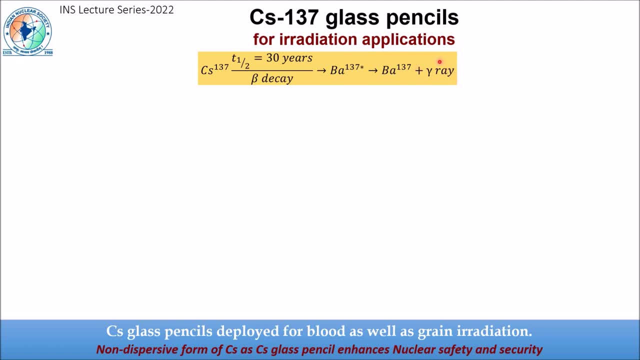 and has a potential application in various gamma irradiation applications. So if we can recover cesium-137 from high-level waste and can convert it into the non-dispersive glass pencil foam as a sealed source, then this sealed source can be utilized for. 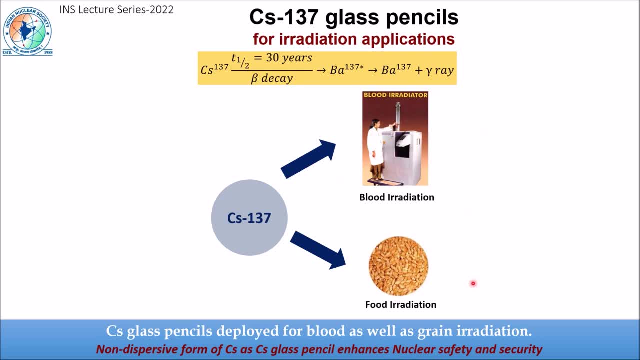 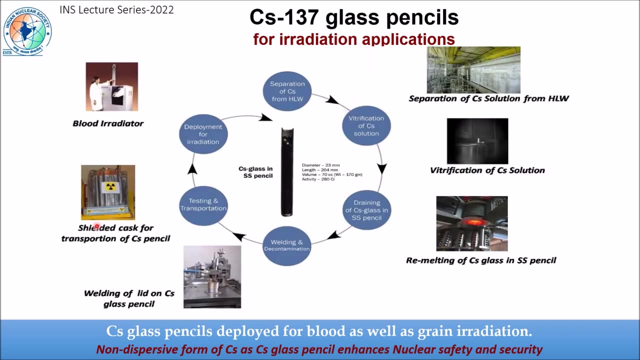 blood irradiation as well as food irradiation. Now let us see how the cesium-137 is recovered from high-level waste in purified form and converted into the non-dispersive glass foam containing sealed source. So, first of all, the cesium is recovered from high-level waste. 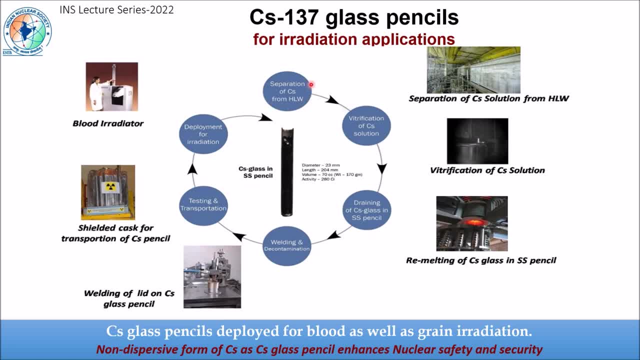 using solenoid extraction based partitioning process, utilizing a spatially designed and formulated extractor which is very selective to the cesium. Thus recovered cesium is then converted into the glass matrix using vitrification process, and then this vitrified cesium 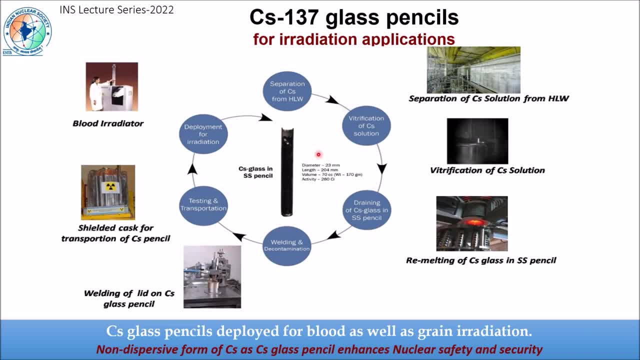 is drained into small stainless steel pencil having a diameter of around 225 mm, having a diameter of around 25 mm and a height of around 200 mm. This stainless steel pencil containing cesium in a non-dispersive glass foam is then remotely sealed. 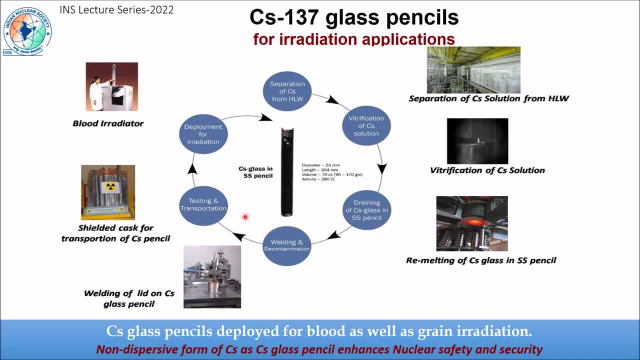 and subjected to the various quality assurance test. After clearing the quality assurance test, this sealed source containing cesium in non-dispersive glass foam is supplied to various hospitals for the blood irradiation application. The recovery of cesium-137 from high-level waste. 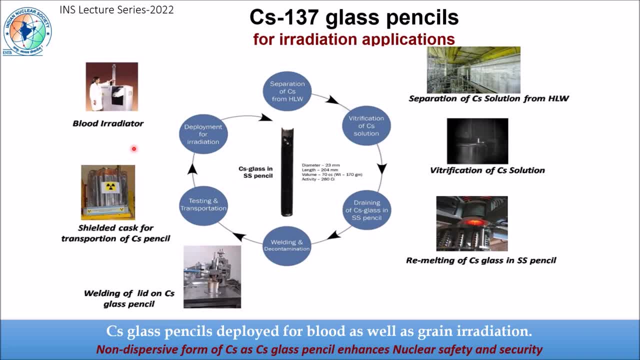 and converting into the non-dispersive glass foam based sealed source adds additional safety to the sealed source. The non-dispersive form of glass will not allow cesium to be dispersed, So cesium-137 was earlier considered as a hazardous radionuclide. 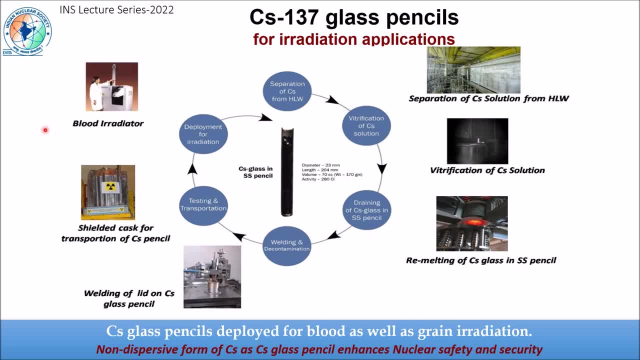 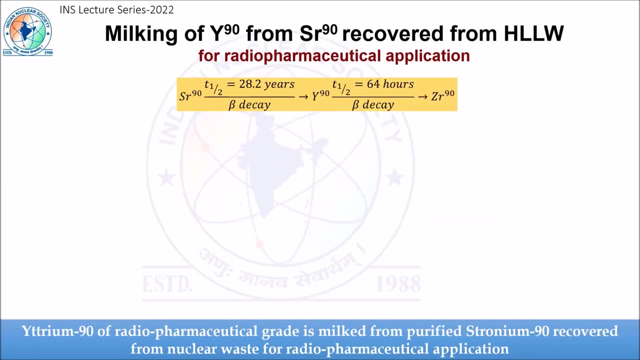 in waste now can be converted into the non-dispersive sealed source and can be utilized for societal application, such as blood irradiation and food irradiation. This is another prominent fission product present in high-level liquid waste, If we see the decay series of strontium-90,. 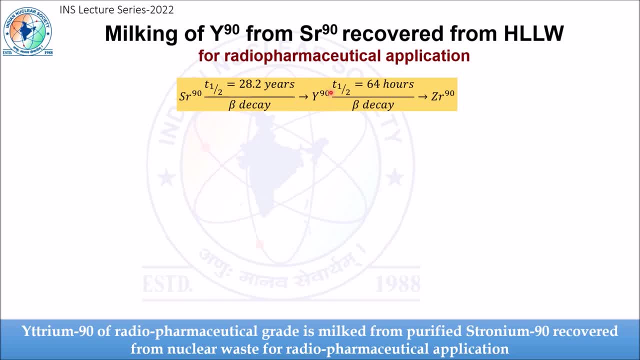 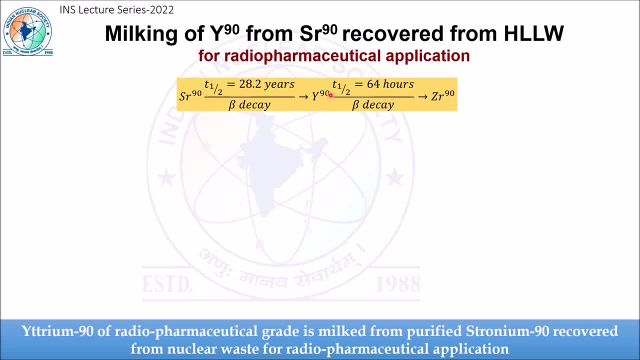 The yttrium-90 is again radioactive in nature, having shorter half-life, finally decays to the stable zirconium-90 product with emission of another beta particle, The beta particle thus emitting out from the decay of yttrium-90. 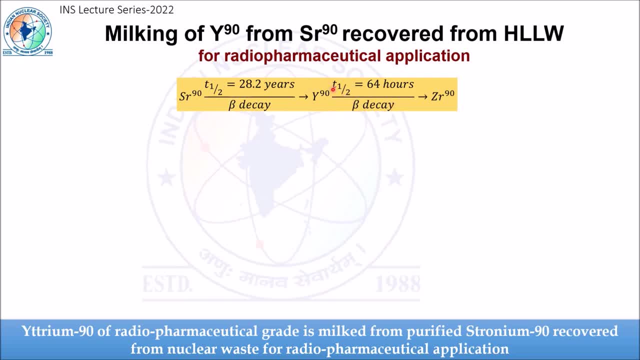 has considerably good energy and has a potential application in radiopharmaceutical requirement. So if we can recover strontium-90 from high-level liquid waste in purified form, the same purified strontium-90 can be utilized for milking of yttrium-90 regularly. 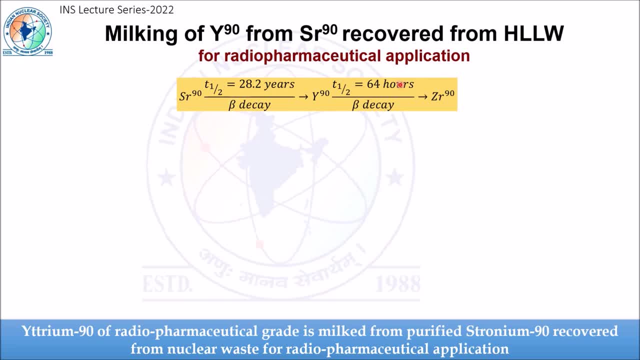 for radiopharmaceutical application. Now let us see how strontium-90 is recovered from high-level liquid waste in purified form and how they are utilized for regular milking of yttrium-90.. So, first of all, the strontium-90 is recovered. 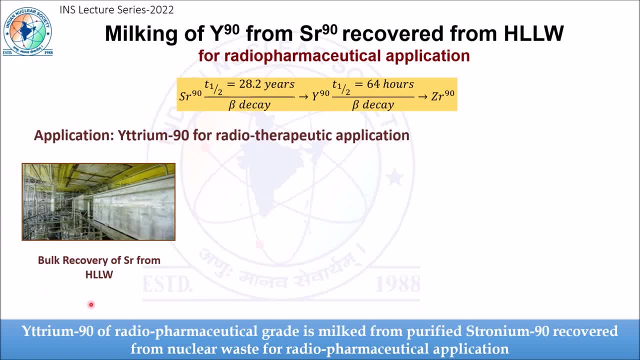 from high-level liquid waste in bulk quantity, again utilizing the solvent extraction method, again utilizing the solvent extraction method, again utilizing the solvent extraction method, and then utilizing the solvent extraction method as it is the active fecalokoloctane at my accelerator solutionに. 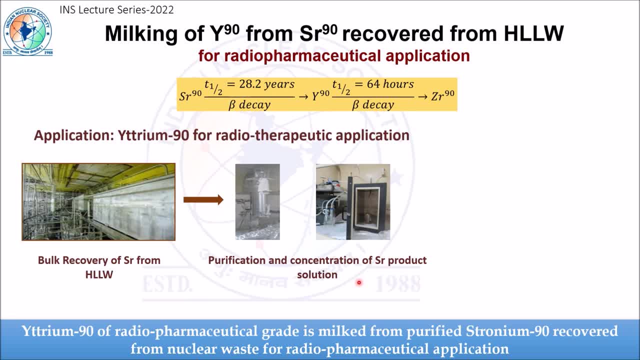 and then utilizing the solvent extraction method, HDMI, of my accelerator solution to anywhere any paternal process, Depending on the type of example, be milked out or recovered from this purified strontium-90 using membrane based techniques and thus recovered or milked out uterium-90 in very purified form, is sent to the hospitals. 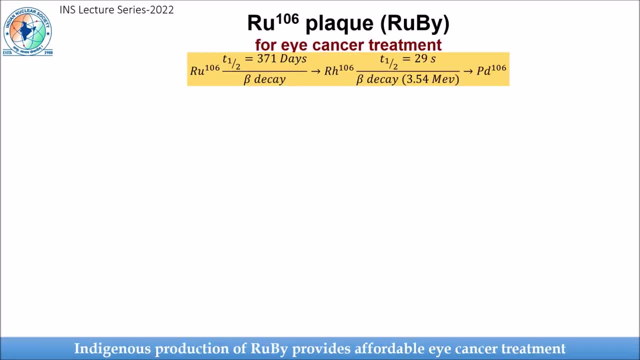 for radiopharmaceutical application. In recent time period, recovery of ruthenium-106 from nuclear waste is demonstrated for its application in eye cancer treatment. Ruthenium-106 decays to rhodium-106, which is also radioactive in nature, having shorter 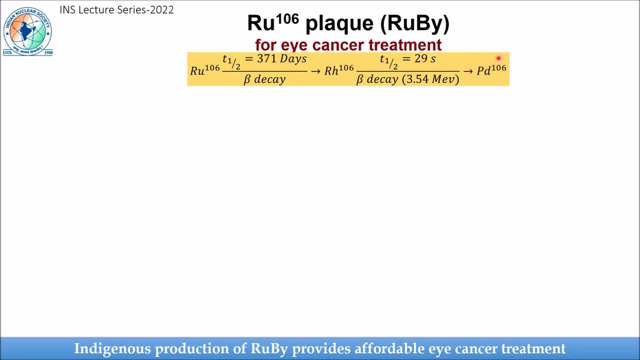 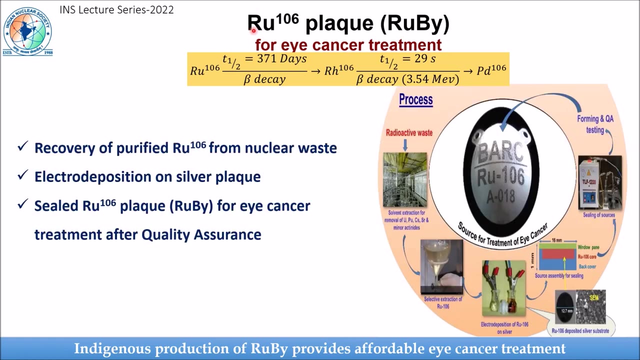 half-life and is further decayed to palladium-106 by emission of beta particle having considerably good energy. This beta particle can be utilized for treatment of eye cancer, Considering the potential of ruthenium-106, recently ruthenium-106- recovery from nuclear. 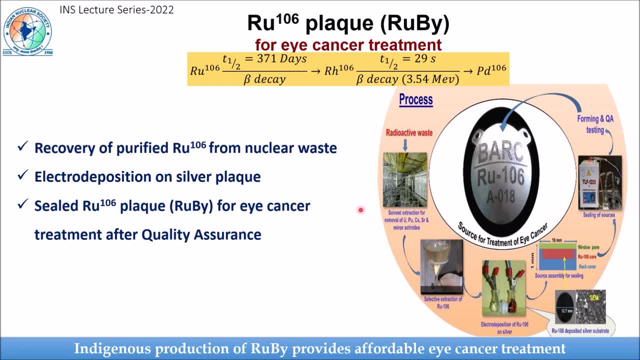 waste has been demonstrated Using solvent extraction as well as other separation techniques, and thus recovered ruthenium-106 is further purified by series of separation techniques, and the purified ruthenium-106 is then subjected to the electro-deposition techniques so that they can be electro-deposited. 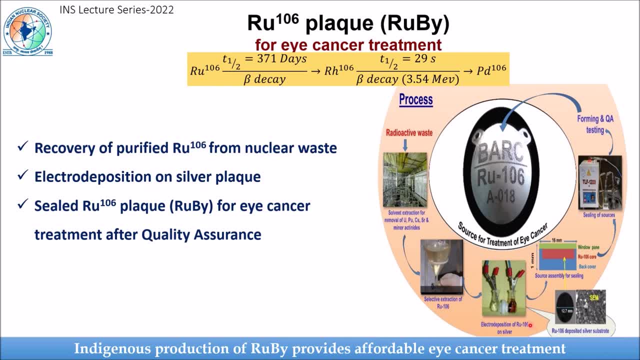 on silver plate. Thus generated ruthenium-106 deposited silver plate is further covered by two another silver plate. The silver plate is then placed on each side and remotely sealed to make a sealed source of ruthenium-106 plague. After ensuring the series of quality assurance test, this ruthenium-106 eye plague can be. 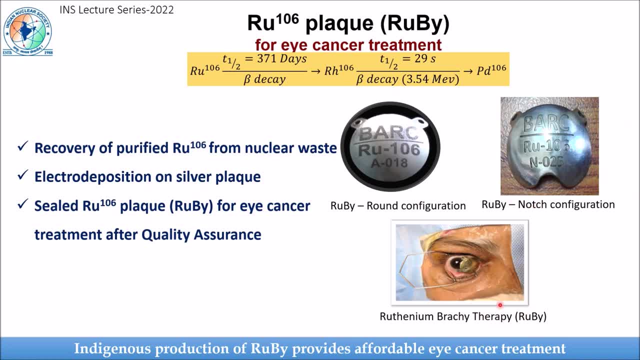 sent to the various hospital for treatment of eye cancer Regularly utilizing the indigenously developed techniques. this ruthenium-106 eye plague can be used for treatment of eye cancer. This ruthenium-106 eye plague can be used for treatment of eye cancer. 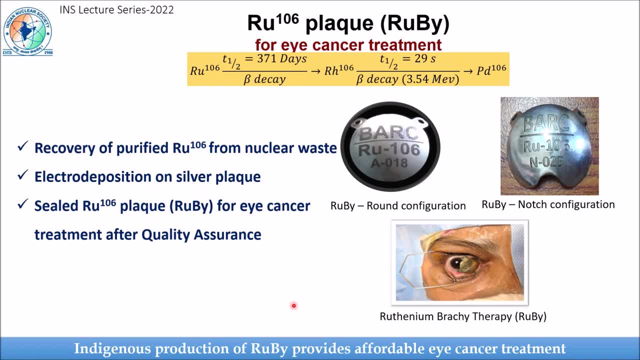 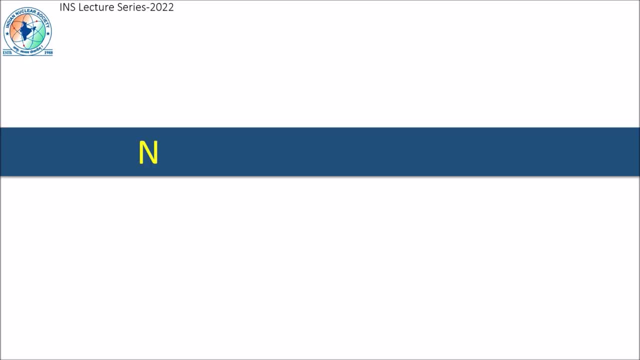 The new technology of radionuclide recovery from nuclear waste is the result of the recent development in the nuclear society. The recovery of valuable radionuclide from nuclear waste could be made possible, and their further deployment in various societal applications converts the nuclear waste into a wealth material. 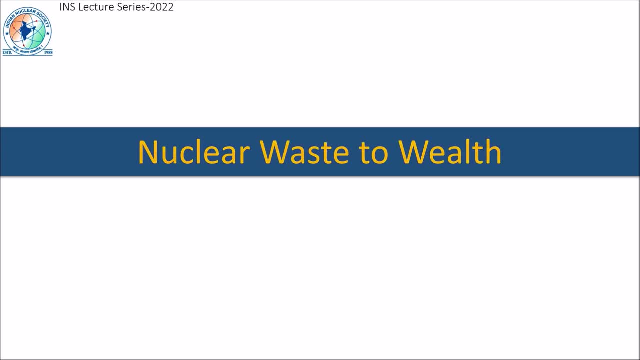 This is the conclusion of this video on this new technology. Thank you, The waste which has been considered earlier as hazardous materials at the moment has been saved and was recovered in the process. This was the solution of the problem. I hope this video was helpful and helpful. 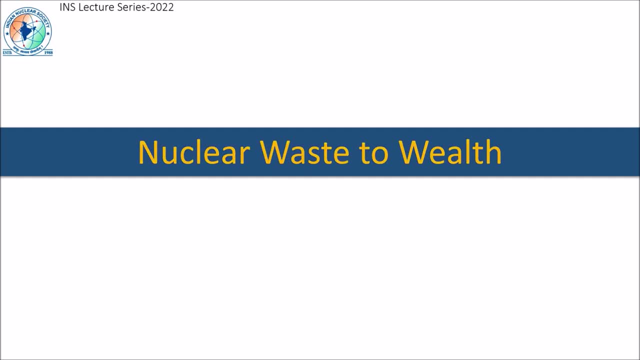 material now is looked as a source of many valuable material, because the nuclear waste is the sole source for many very valuable radionuclides which have various societal applications. So the indigenous development in the field of nuclear waste management and particularly in the field of recovery of valuable radionuclide, not only aims to recovery and reuse. 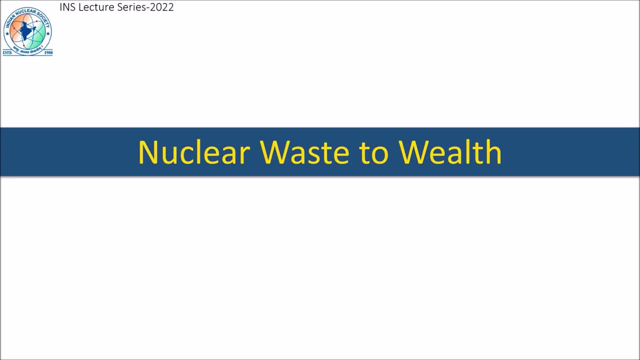 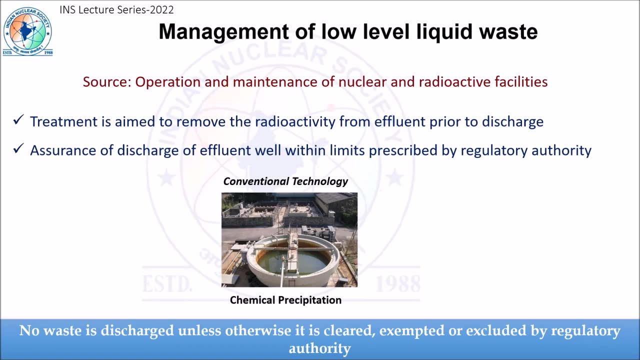 of material, but also a step towards Atmanirbhar Bharat, to make the India self-reliance. Besides spent fuel, operation of nuclear reactor also generates low-level liquid effluents, and this liquid effluents need to be treated safely and efficiently for the removal of radioactivity prior. 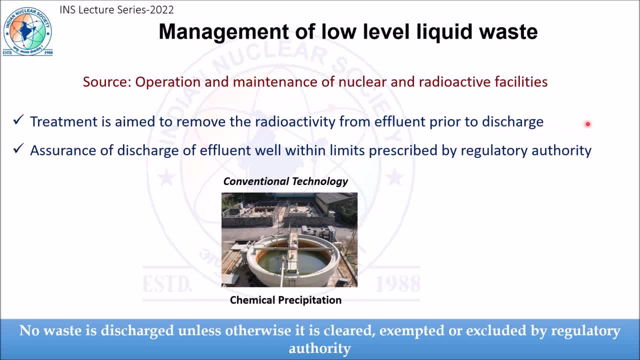 to their discharge. The major challenges related to the treatment of low-level liquid effluents are mainly the following: First of all, the treatment of low-level liquid effluents is a major challenge. Second of all, the treatment of low-level liquid effluents is a major challenge. 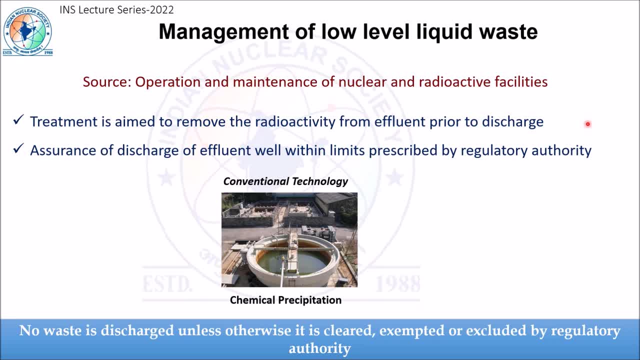 This is mainly due to their associated larger volume and removal of radionuclide which are already present in very, very low concentration in the effluent. Conventionally, chemical precipitation-based technology has been deployed for the treatment of low-level liquid effluent for the removal of radioactivity prior to their discharge, and it has been always. 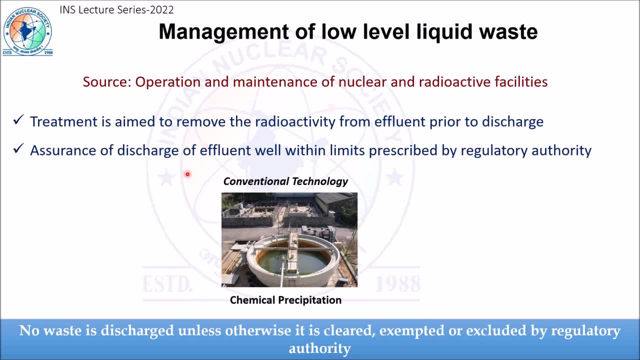 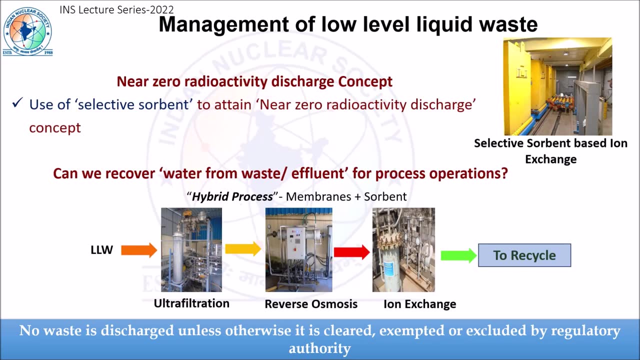 assured that, whatever the effluents are discharged, they should contain the radioactivity well below the limits which are prescribed by the regulatory authority, so that they are not harmful further. But still the question arises: can we attain the concept of near zero discharge of radioactivity? 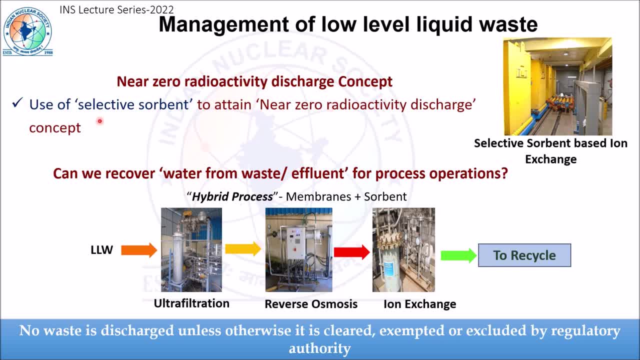 For the same, selective sorbent-based process has been developed and demonstrated for the treatment of liquid effluent, so that the radioactivity from effluent can be reduced to the negligible level prior to their discharge. Besides this, the membrane and sorbent based 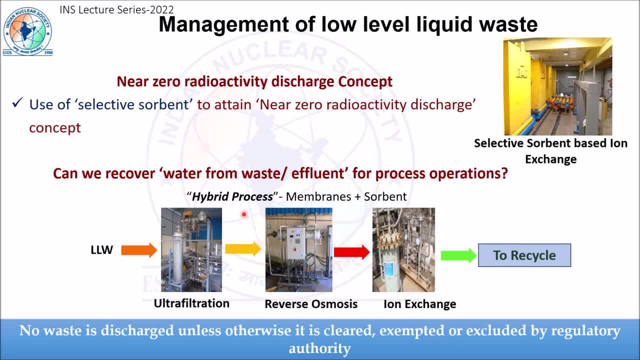 hybrid process has been recently developed and demonstrated for the treatment of liquid effluent aiming towards the removal of radioactivity to such a level that the treated waste coming out from the process has a very, very, very low amount of, or negligible amount of, radioactivity. and same can be высокly. Swifted flux constantlyası 60 % trouble the job of a added dose to theання for immediate disposal in the buyers projector to such a level that treated waste coming out of the process as a way very, very, very low amount of negative amount of radioactivity and same can be 크 to reach, reach fridge by the mehr weapons of nuclear enterprises as possible. 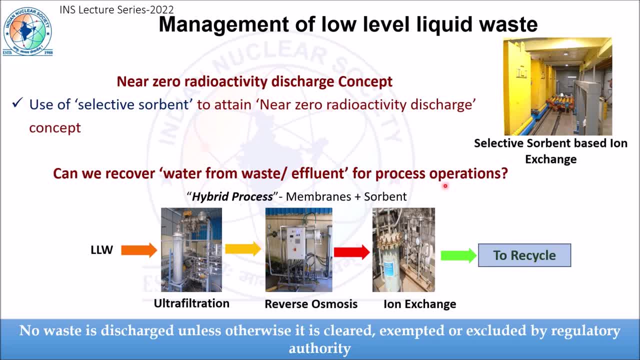 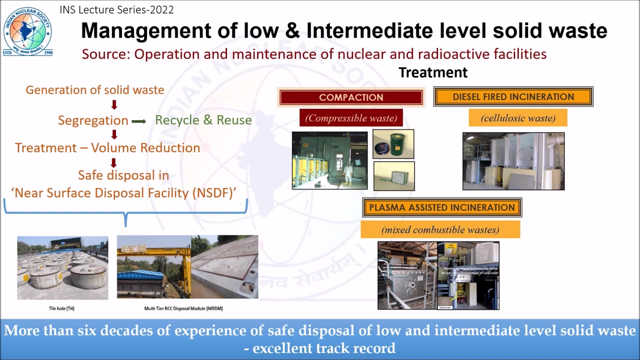 can be recycled back for various process operation. So demonstration of such hybrid process helps us in realizing the recovery of water from the waste, which is an important step towards the water conservation. Operation of nuclear reactor and associated fuel cycle facilities also generate radioactive solid waste. As a first step towards the management of these radioactive solid 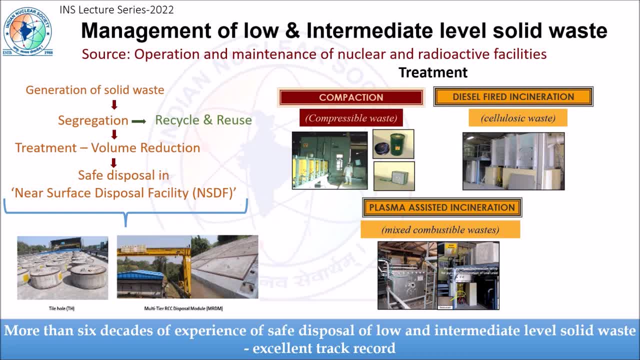 waste. the waste is segregated properly so that the recycle and reuse of the material can be assured as far as possible. The remaining waste is then treated using various volume reduction techniques, including compaction and incineration techniques, so that the final waste volume can be reduced. 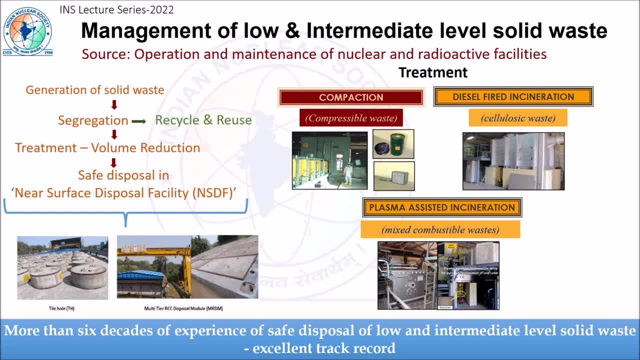 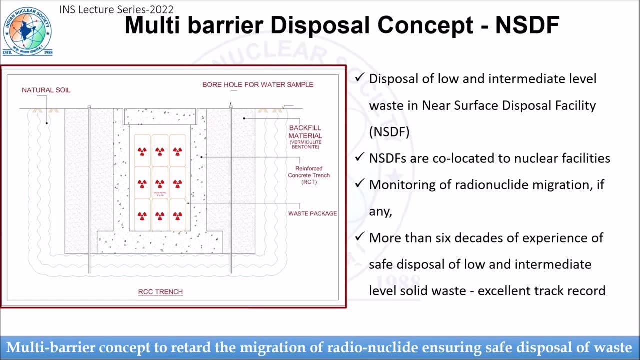 effectively. These wastes are then conditioned or immobilized in a cement matrix, and then they are safely disposed in near surface disposal facility, which is conventionally called as a NSDF. The NSDFs are specially designed and constructed based on the multi-barrier disposal concept, which is the 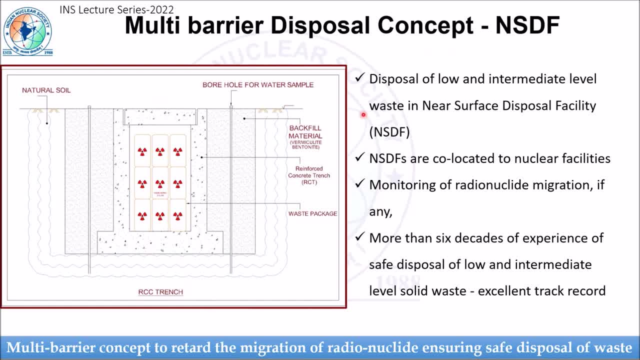 combination of various engineered barriers and natural barriers. So when conditioned waste is disposed in NSDF, the series of engineered barriers and natural barrier do not allow the migration of the radionuclide from this waste. In India we have more than six decades of experience of treatment and safe. 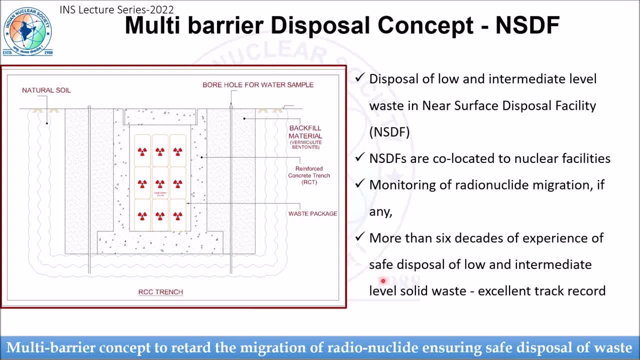 disposal of radioactive solid waste in NSDF with an excellent track record. We have already seen that the nuclear energy generates lesser amount of the waste volume, and the same can be further illustrated based on the requirements of the space for NSDF for the disposal of solid waste. 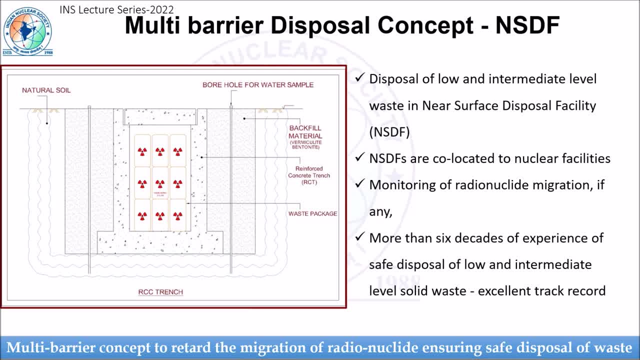 The capacity of nuclear power plant in India. if it can continue to be operated for next 50 years, then whatever the radioactive solid waste is getting generated that can be safely disposed in NSDF having size of only a cricket ground. This further strengthens our understanding. 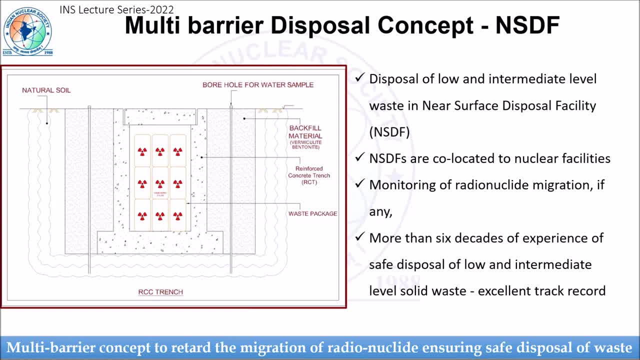 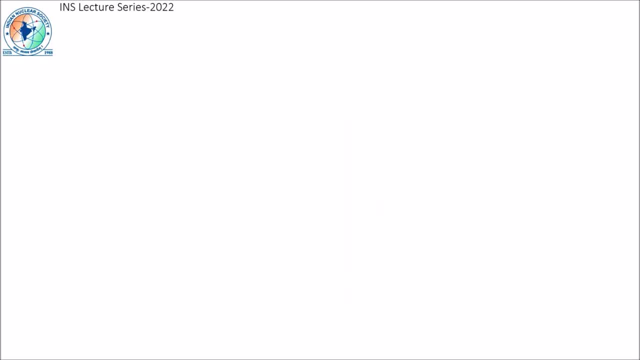 that nuclear energy generates lesser amount of waste volume. So now let me summarize the complete lecture in few sentences, and the first and most important is: the highest priority has been given to the safe management of nuclear waste since inception of nuclear power program in our country. As a result, we do have more than 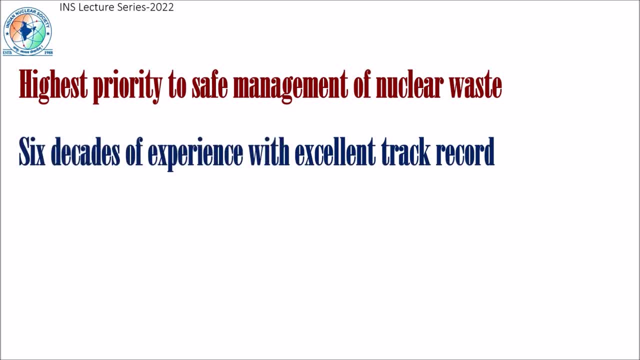 six decades of experience in the nuclear industry in the field of management of nuclear waste, with excellent track record. With ongoing R&D, various new technologies have been developed which are not aiming to only to the waste volume minimization, but also trying to attain the concept of near zero discharge of activity. 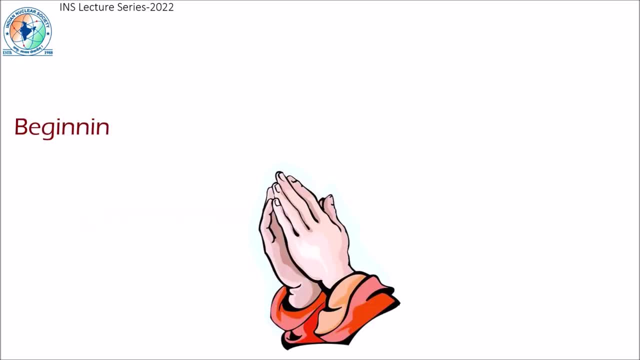 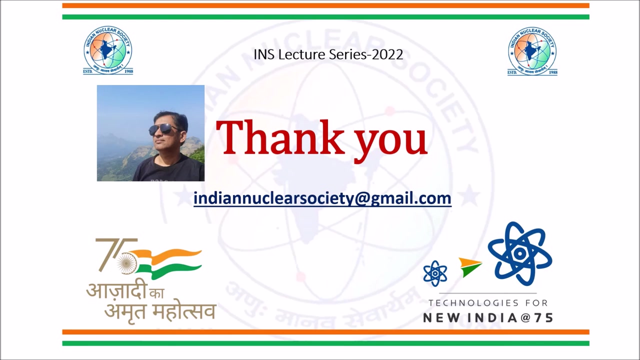 and also to recover the valuable radionuclide from nuclear waste for their deployment in various societal applications to realize the concept of wealth from nuclear waste. So I hope you all enjoyed this lecture. Do not miss other lectures from Indian Nuclear Society. If you have any questions, please write to us on this email id. Thank you.